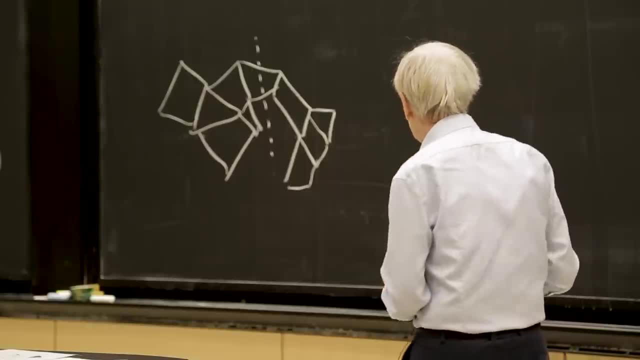 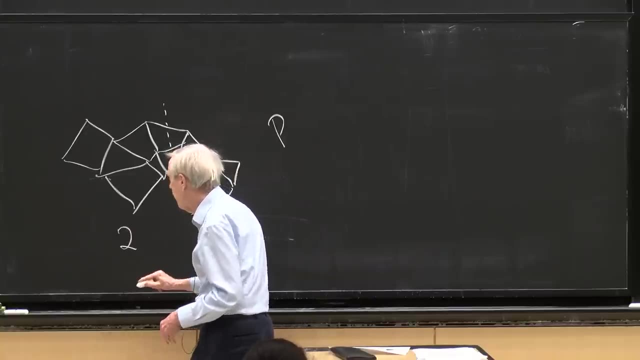 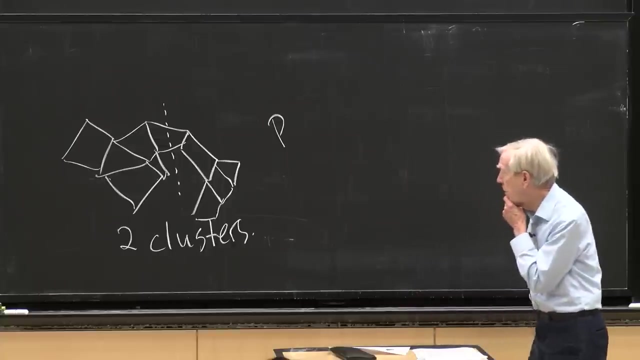 What's an algorithm that would find that cut? So that's a problem. Let's say we're looking for two clusters. We could look for more clusters, But let's say we want to look for two clusters. So what are we trying to do? 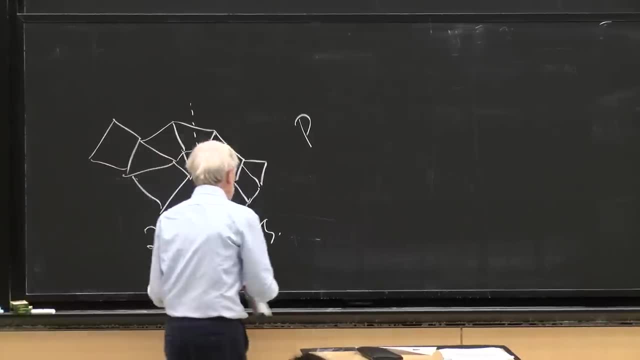 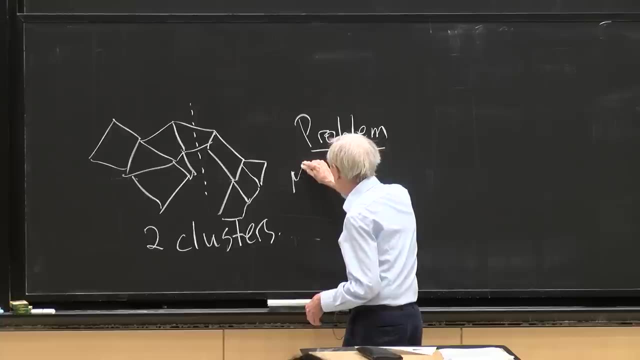 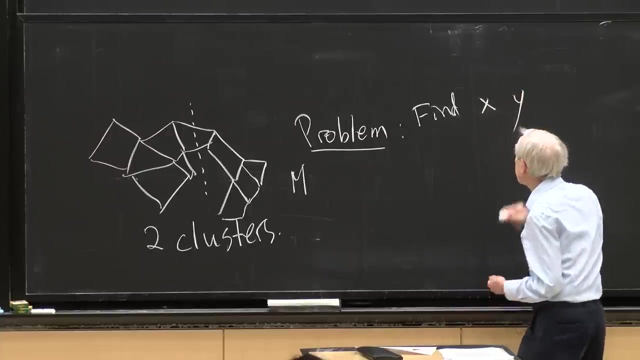 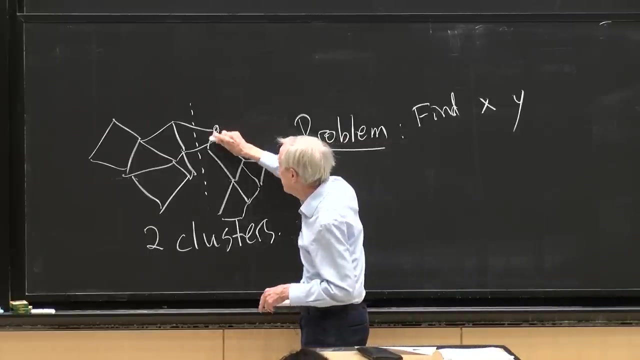 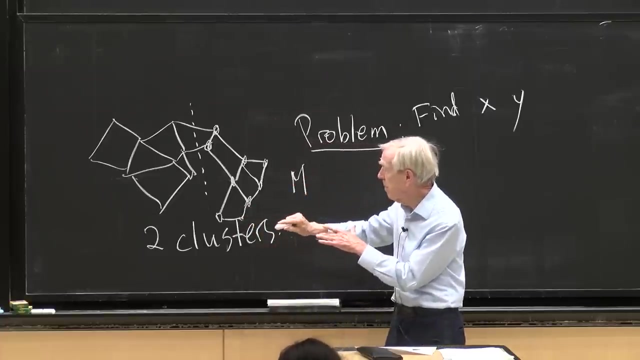 We're trying to minimize. So this is the problem then. So we look for, find positions x and y, let's say, which will be the center, so to speak, of the, And really it's just these points. So the data is the points and the edges, as always. 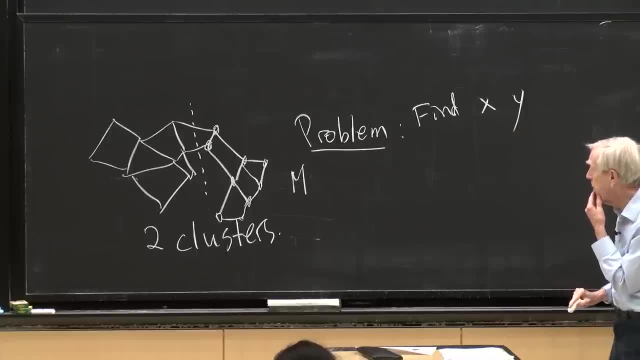 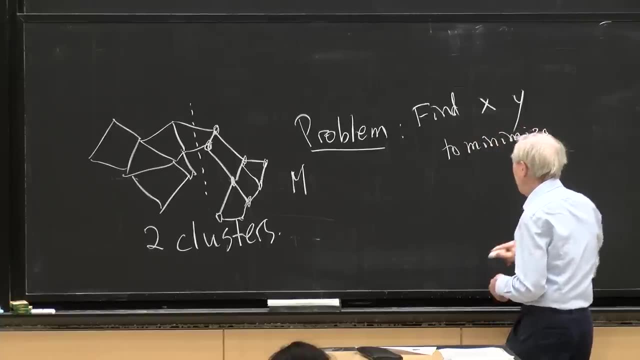 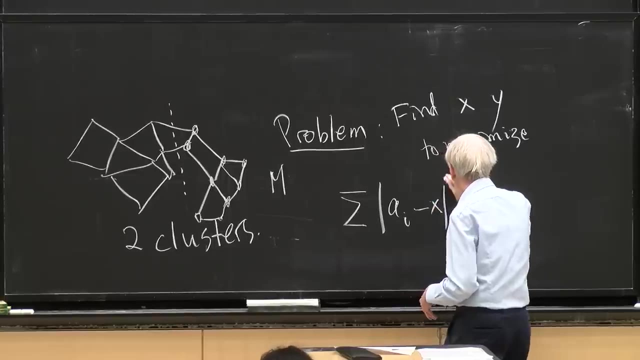 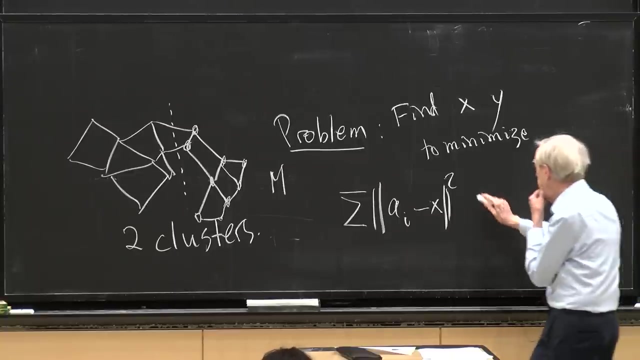 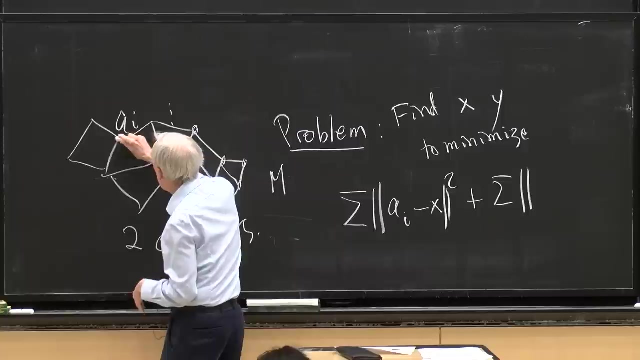 the nodes and the edges. So the problem is to find x and y so that to minimize- so it's a distance of points, ai from x maybe should emphasize- we're in high dimensions- plus the distance from other points. So the ai will be these points, these nodes. 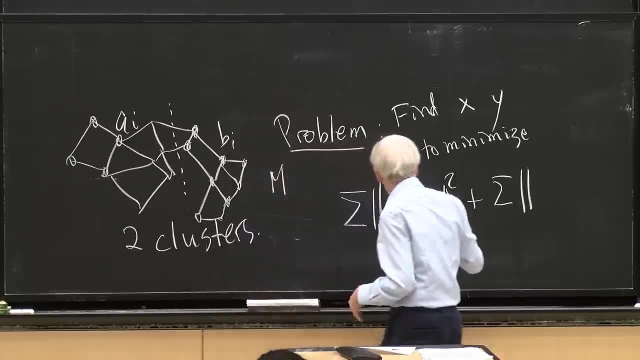 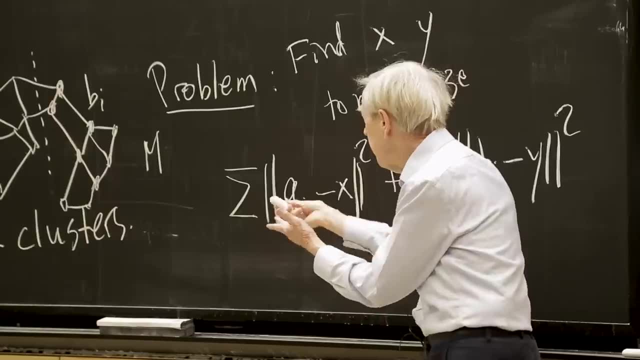 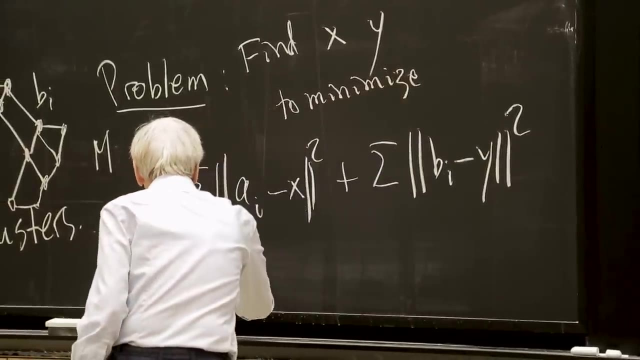 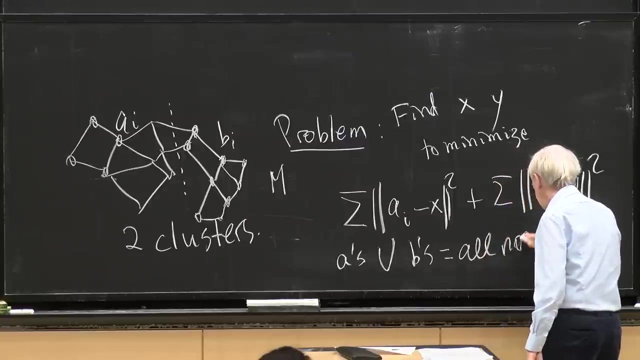 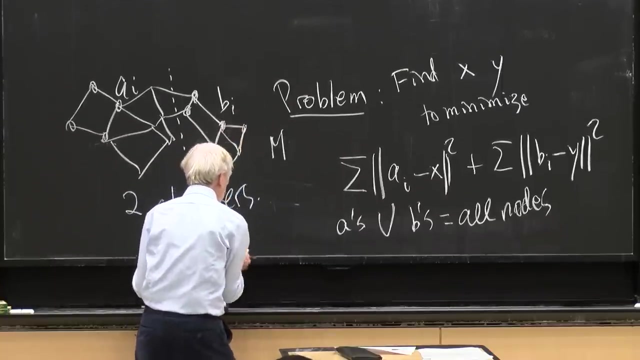 and the bi will be these nodes plus the sum of bi minus y squared, And you understand the rule here that together, the A's union, the B's give me all nodes And I guess, to be complete, the A's intersect, the B's is empty. 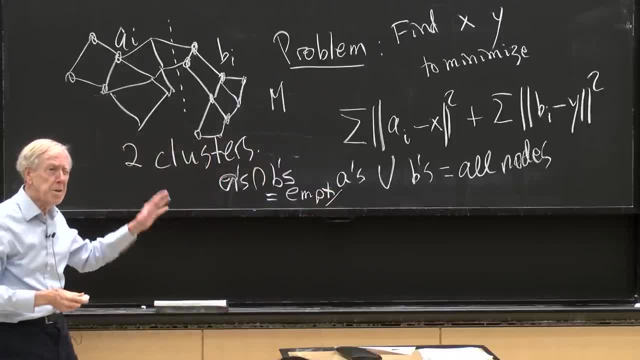 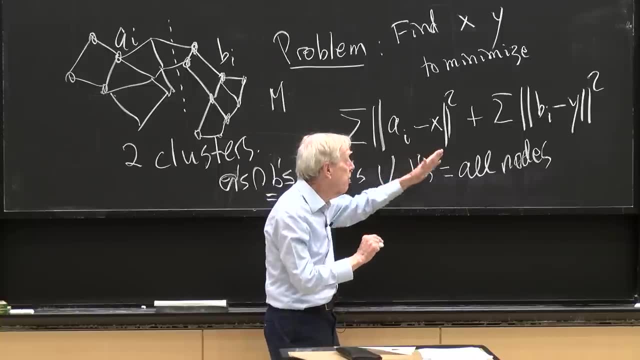 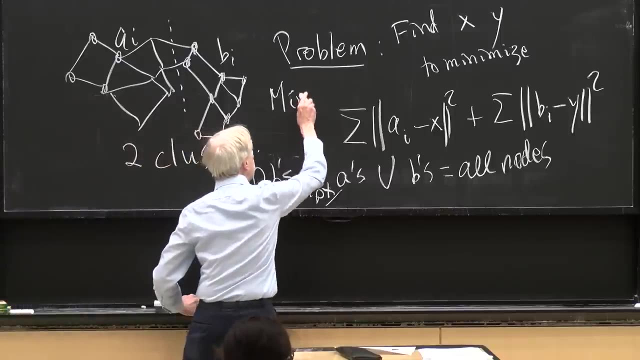 Just what you expect. I'm dividing the A's and the B's into two groups And I'm picking an x and a y, sort of at the center of those groups, so that that is a minimum. So I want to minimize And also I probably want to impose some condition. 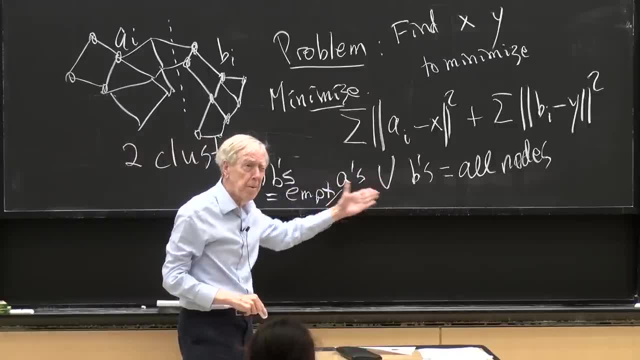 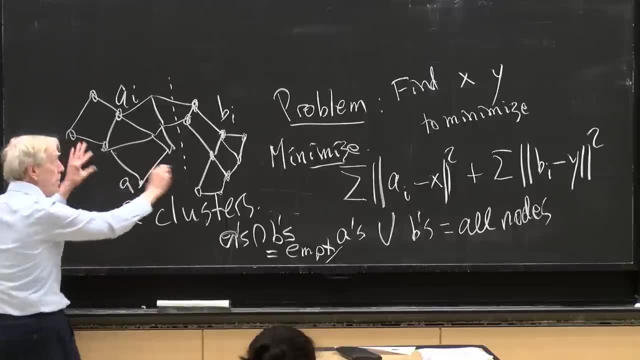 that the number of A's is reasonably close to the number of B's. In other words, I don't want, I just want that to be the A and all the rest to be the B's. That would be not a satisfactory clustering. 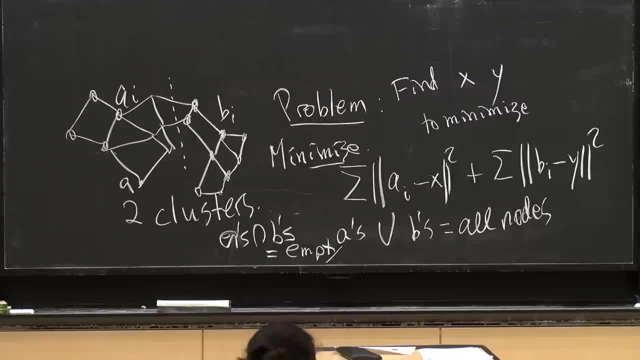 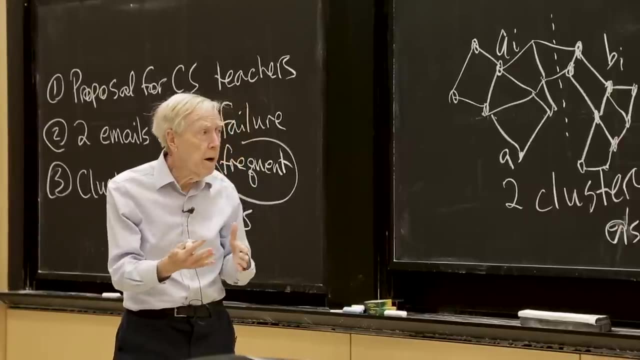 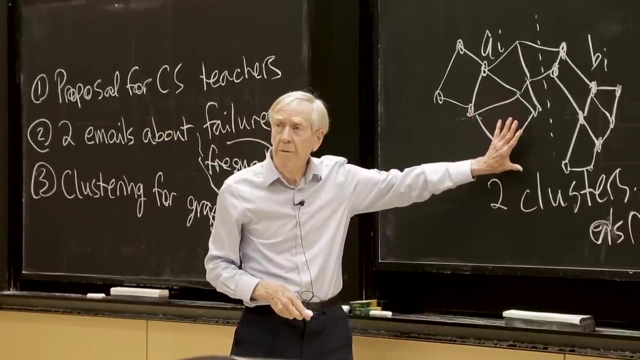 I'm looking for clusters that are good sized clusters, So minimize that, OK. So there are a lot of different algorithms to do it. Some are more directly attacking this problem. Others use matrices that we associate with the graph. So let me tell you about two or three of those algorithms. 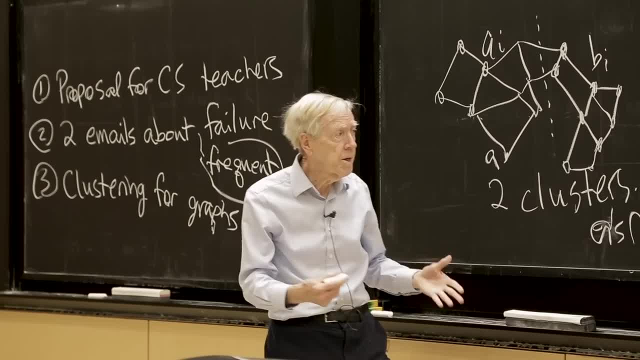 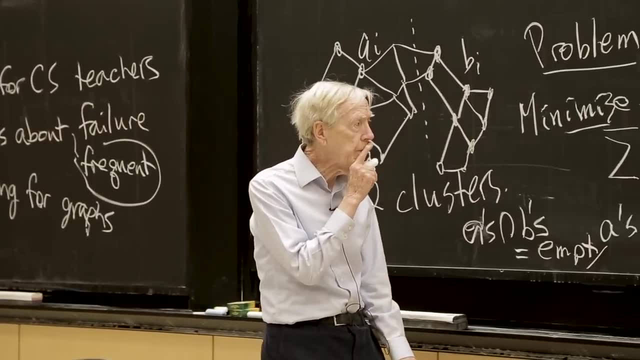 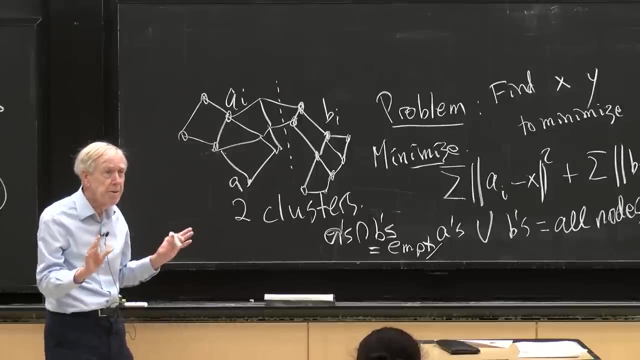 And if you've studied, had a course in graph theory, you may already have seen this problem. First question would be: suppose I decide these are the A's and those are the B's, or some other decision? Yeah, probably some other decision. 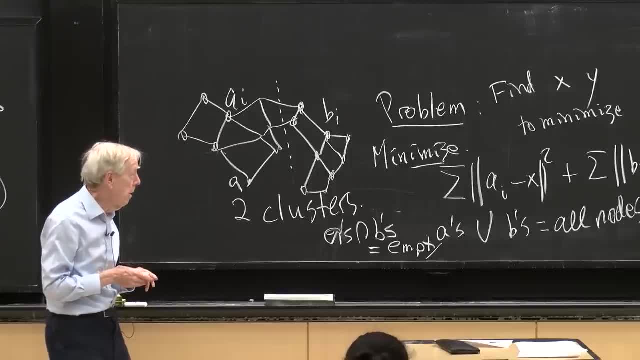 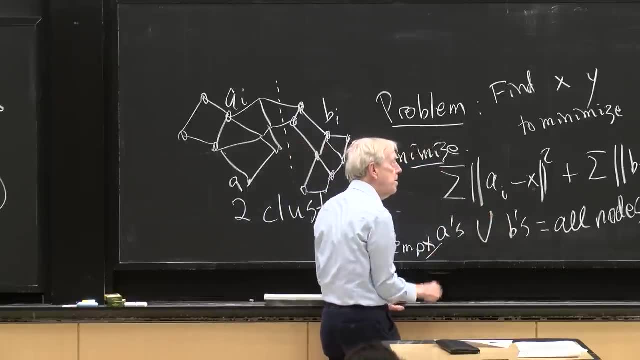 God, don't want to solve the problem before I even start, Sorry. So some A's and some B's. What would be the best choice of the X, once you've decided on the A's, And what would be the best choice of the Y? 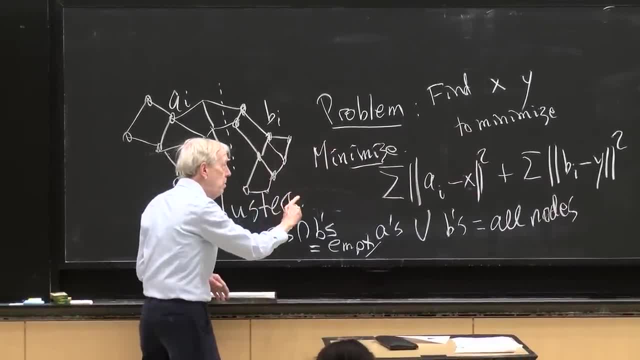 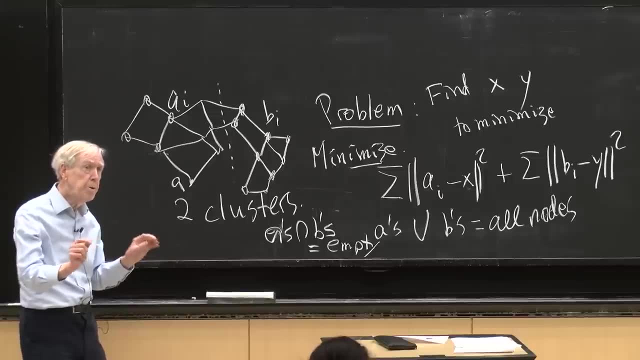 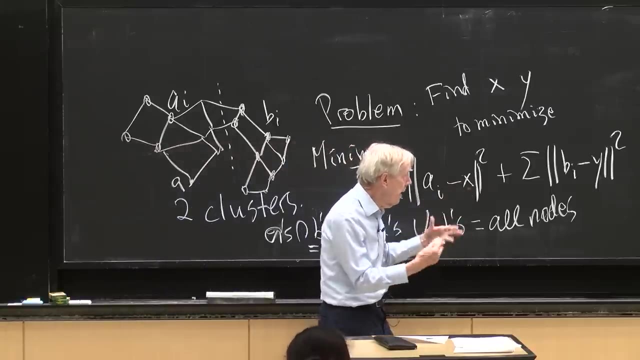 once you've decided on the B's So we can answer that question. Just if we knew the two groups, we could see where they should be centered, with the first group centered at X, the second group centered at Y. And what does centering mean? 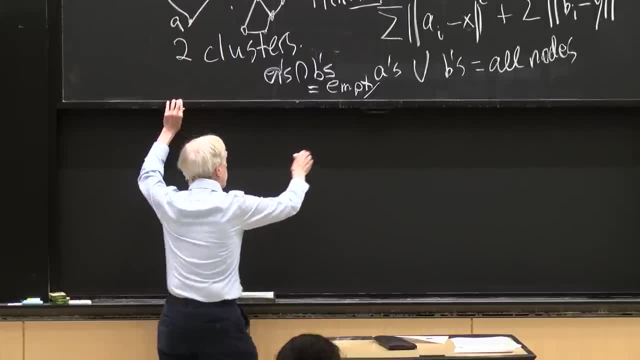 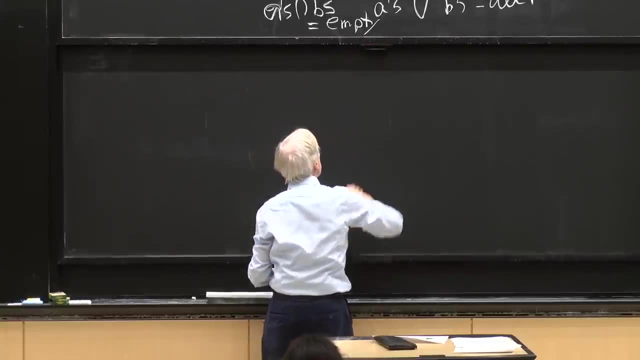 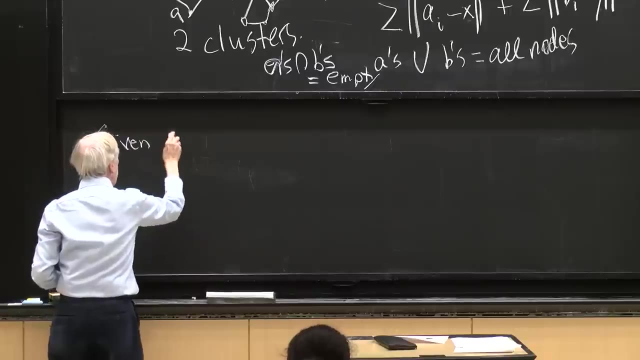 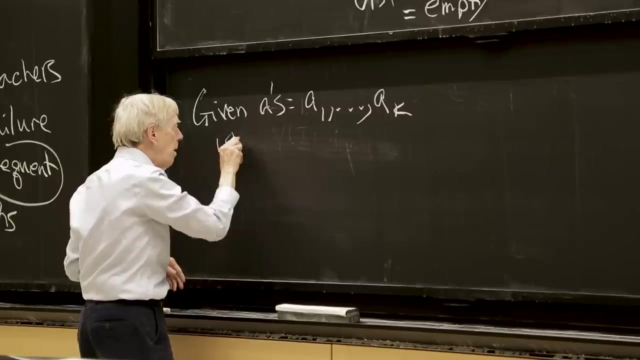 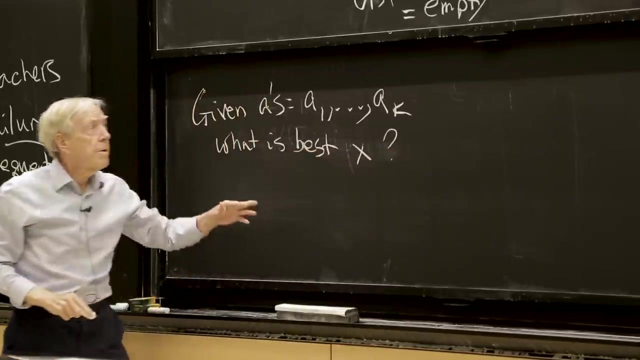 So let's just say so. I think what I'm saying here is- let me bring that down a little- So, given the A's, this is A1, up to say AK. what is the best is the best? X, just to make that part right. 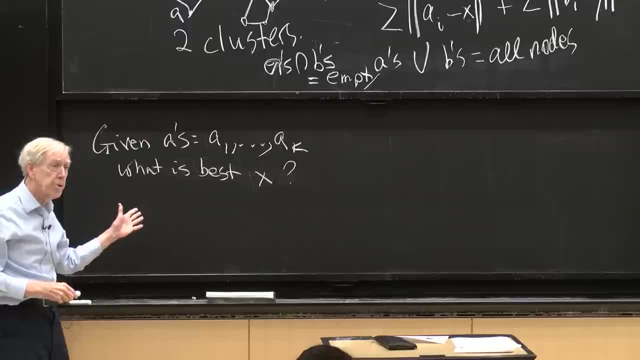 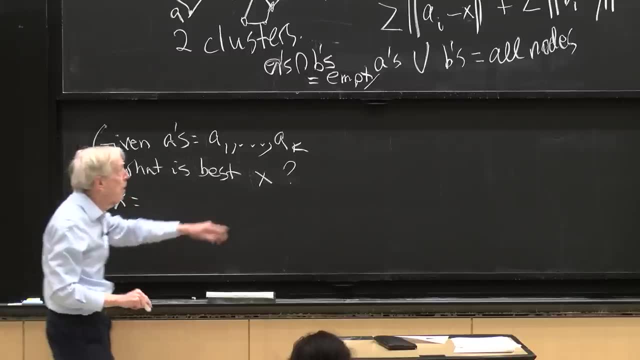 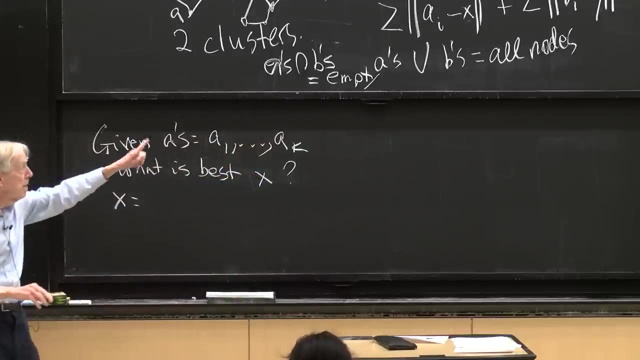 And the answer is: do you know geometrically what X should be here? X is the. so if I have a bunch of points and I'm looking for the middle of those points, the point X, a good point X, to say, OK, that's the middle. 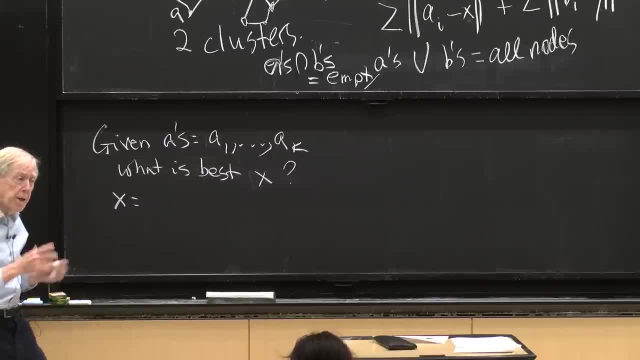 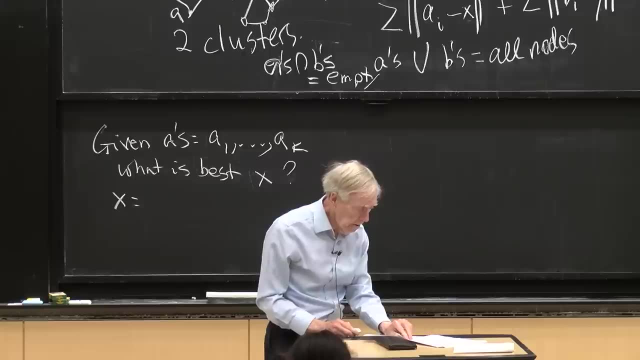 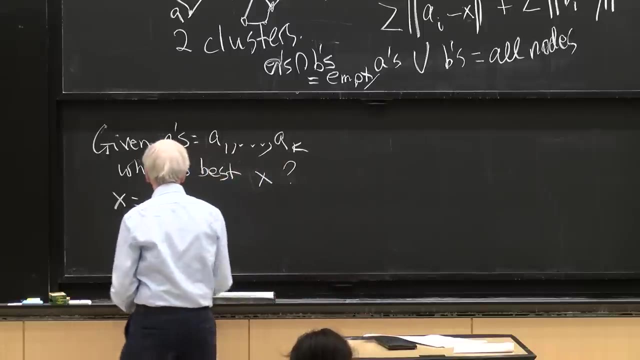 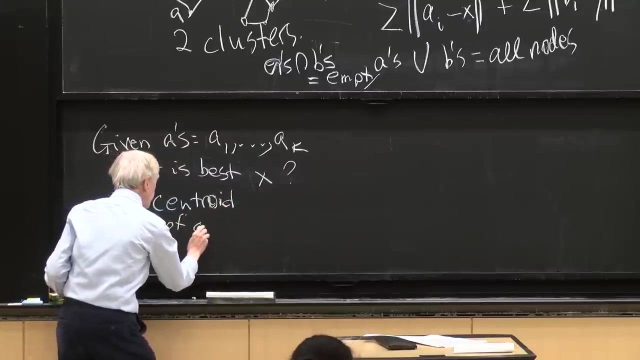 It'll make the sum of the distances- I think, square, And I hope I'm right about that- a minimum. What is X? It is the centroid. Centroid is the word, X is the centroid of the A's. And what is the centroid? 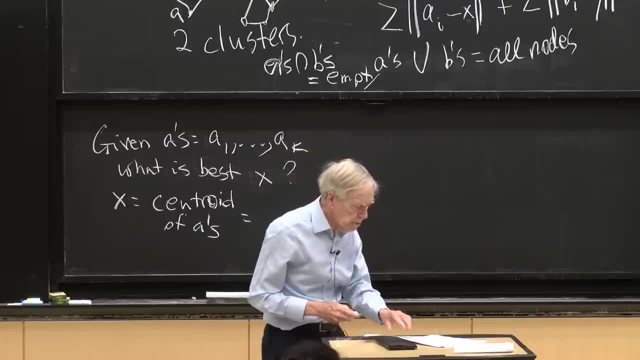 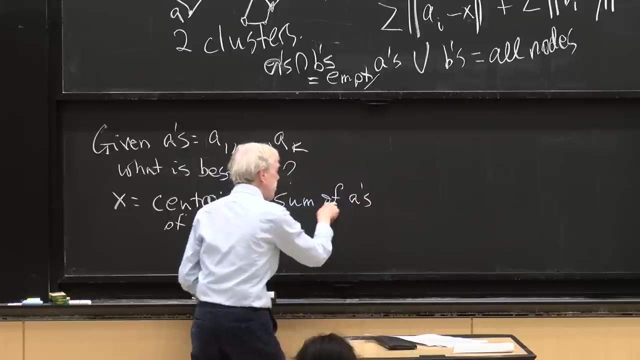 Let's see. Oh, maybe I don't know if X and Y were a good choice, but Let me see what I guess it's the average A, It's the sum of the A's, of these A's- Those are vectors, of course- divided by the number of A's. 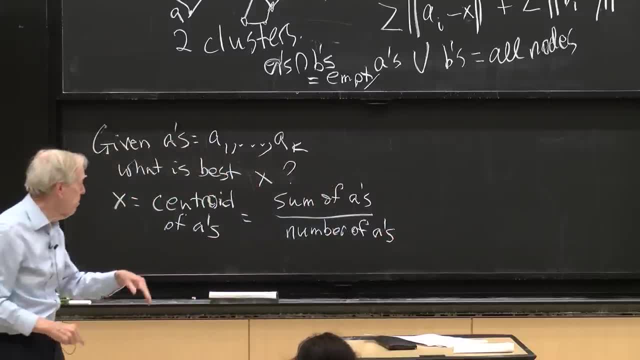 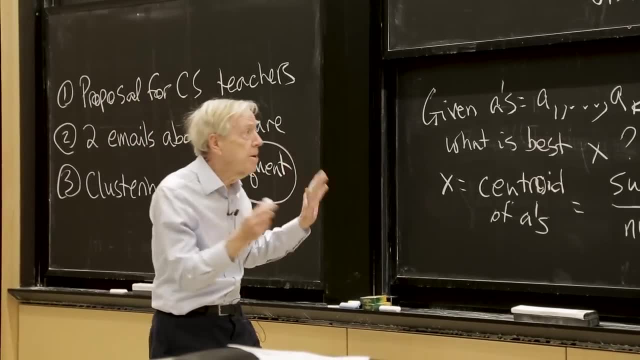 I think. Actually, I was just quickly reviewing this morning, so I'm not totally on top of this Centroid. What I'm going to talk, the algorithm that I'm going to talk about, is the K. well, K means 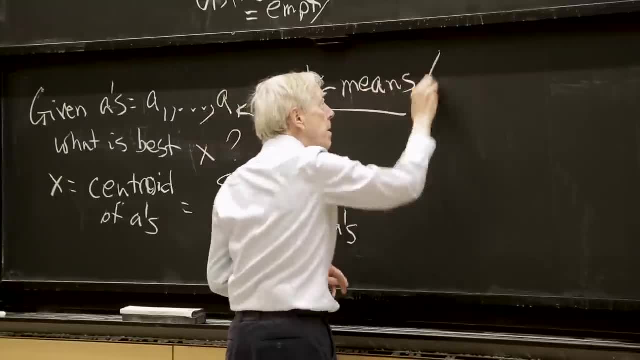 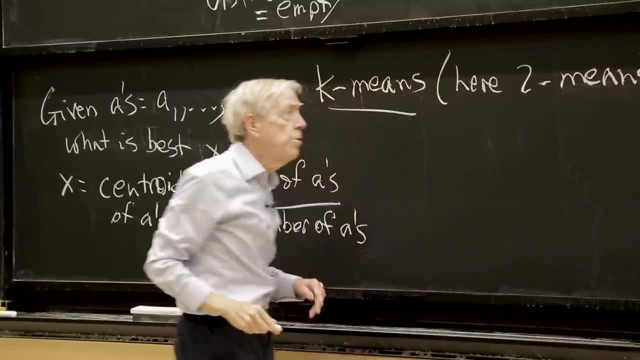 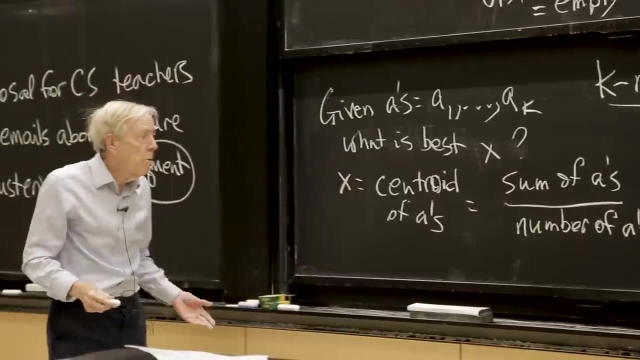 it's always called, And here it will be, the K will be 2.. I just have two partitioning into two sets, A's and B's, So I just K is just 2.. OK, what's the algorithm? 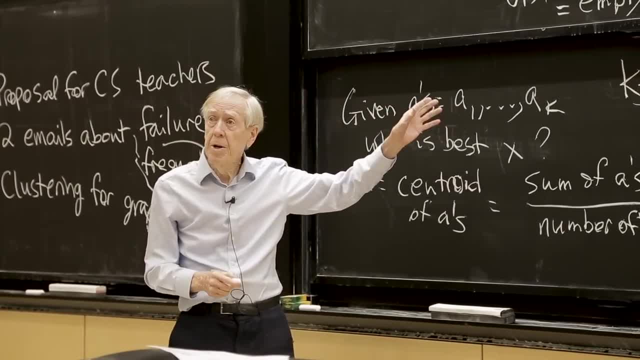 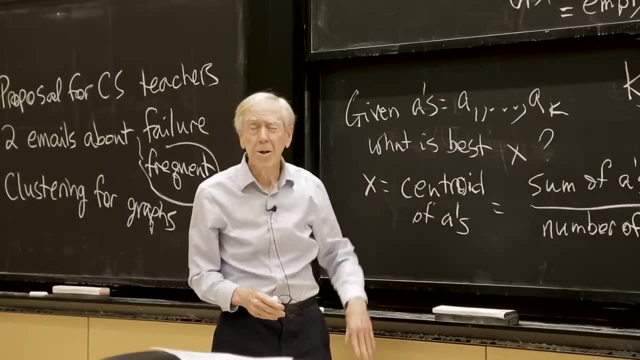 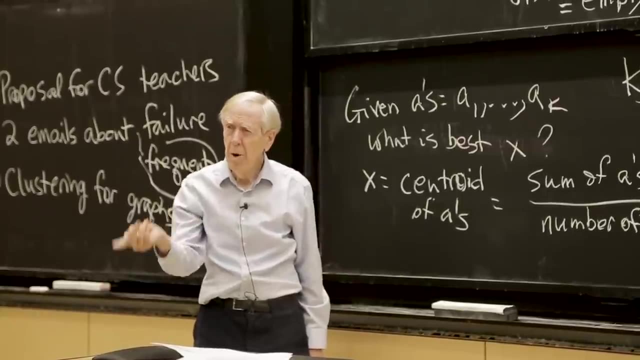 Well, If I've chosen a partition, the A's and the B's have separated them, then that tells me what the X and the Y should be. But now what do I do next? So this is going to be a sort of an alternating partition. 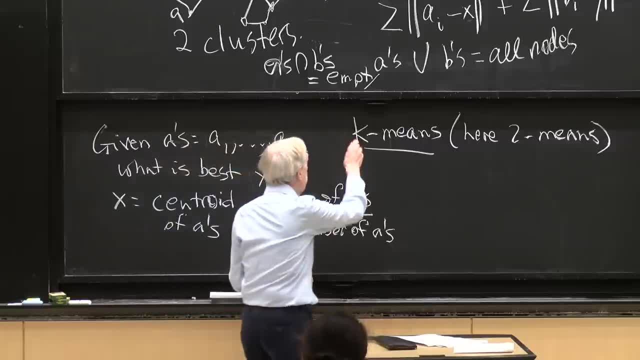 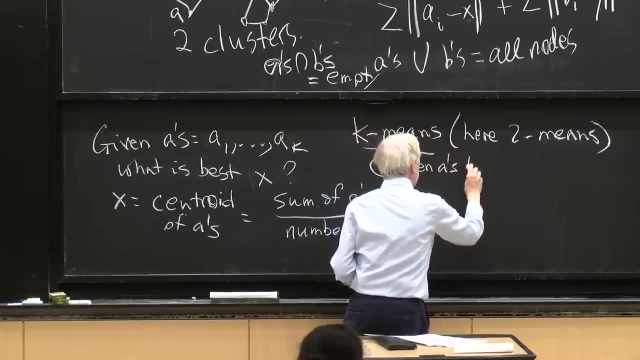 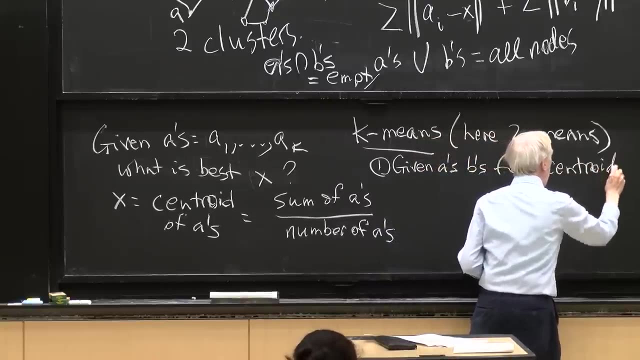 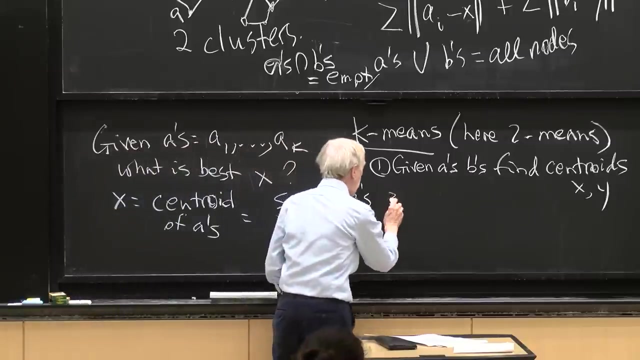 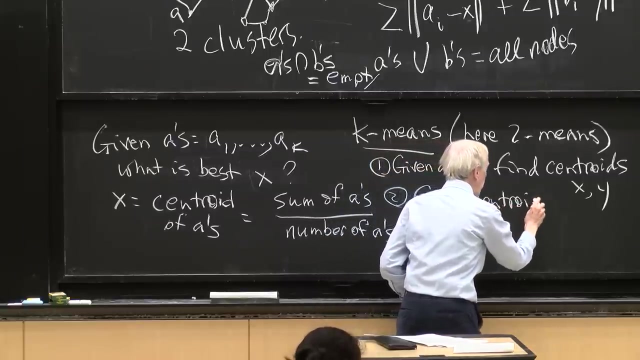 Now I take those two centroids. So step one is for given A's and B's. I'm going to do this. These find the centroids X and Y, And that's elementary. Then the second step is: given the centroids X and Y. 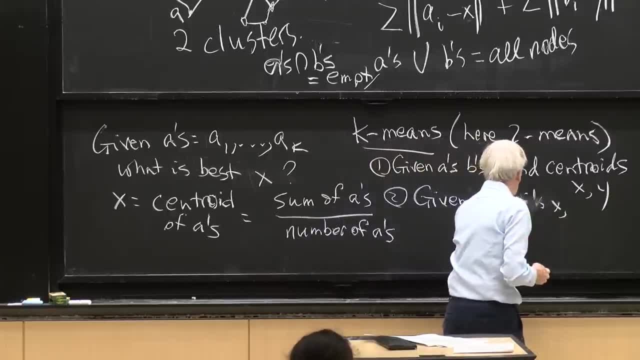 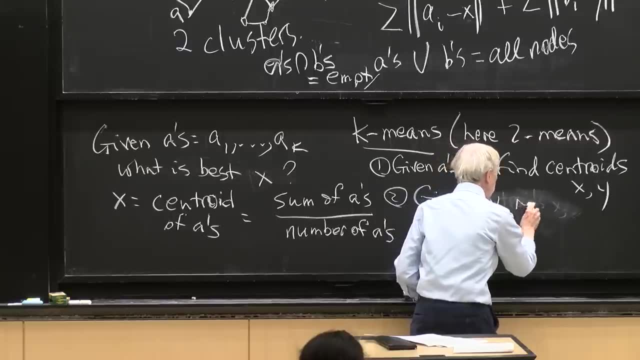 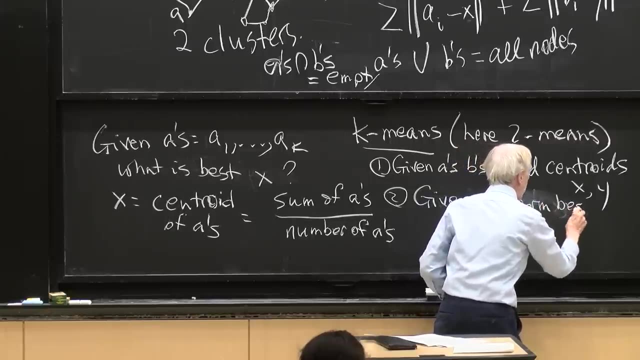 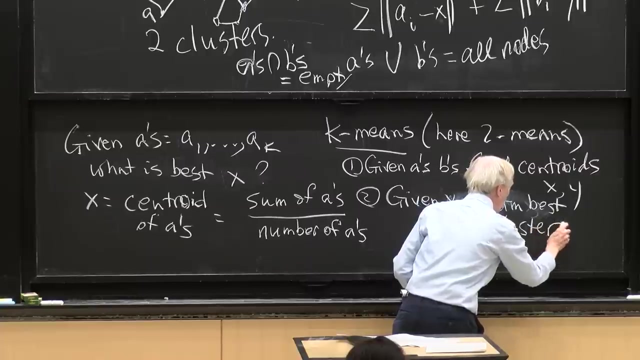 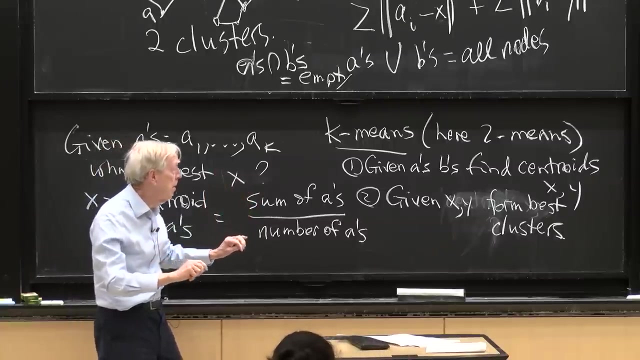 given those positions, given X and Y, they won't be centroids. when you see what happens, Given X and Y, re-form, the best partition, best clusters. OK, so step one: we had a guess at what the best clusters were. 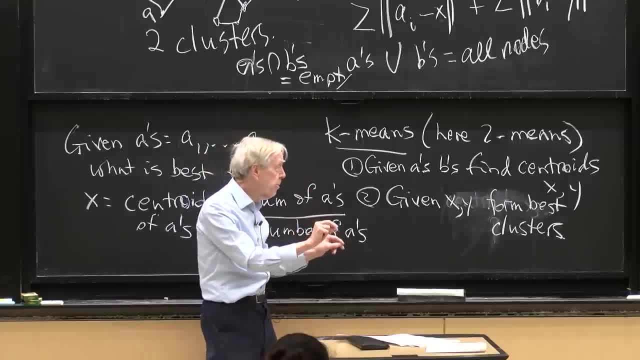 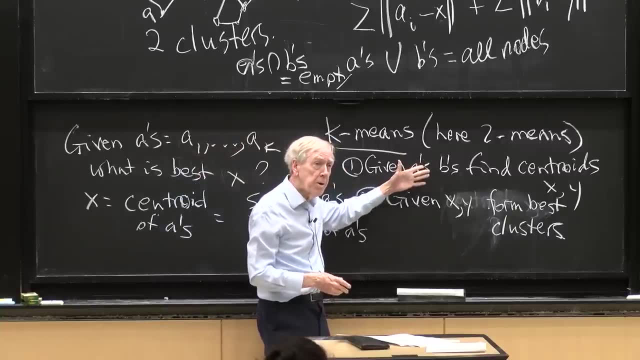 And we found they're centroids. Now we start with a centroid, Now we start with a centroid, Now we start with a centroid And we form new clusters again, And if these clusters are the same as the ones we started with, then the algorithm is converged. 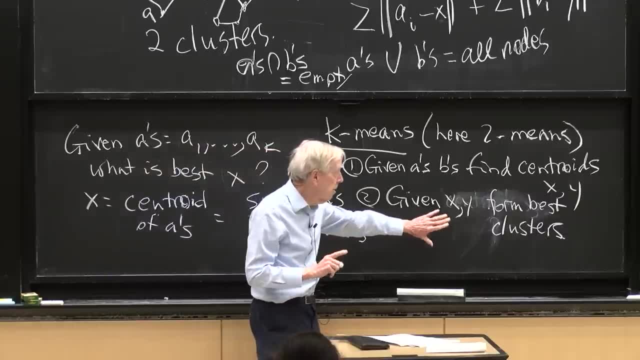 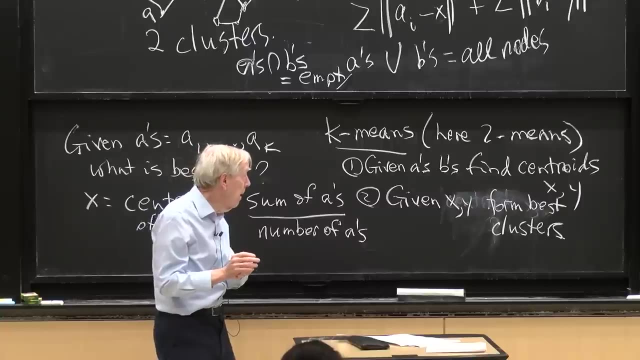 But probably won't be these clusters. So you'll have to tell me what I mean by the best clusters. If I've got the two points X and Y, I want to separate all the points that cluster around X to the ones that cluster around Y. 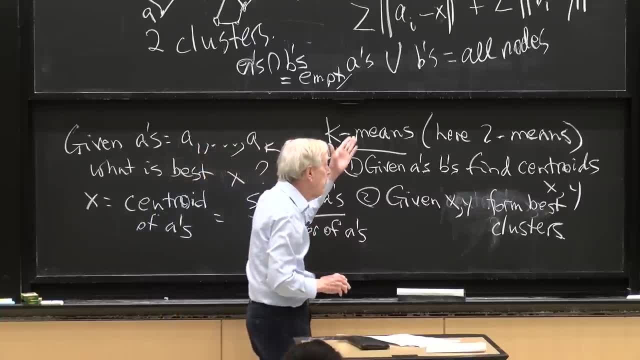 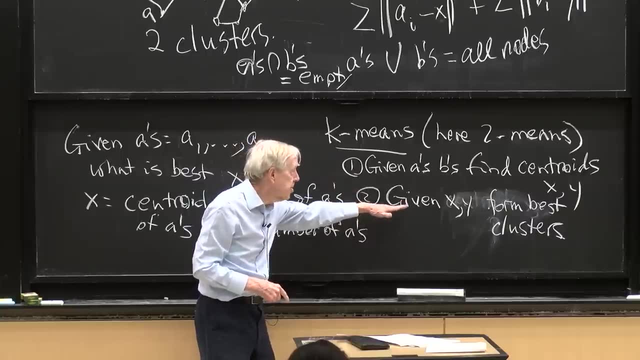 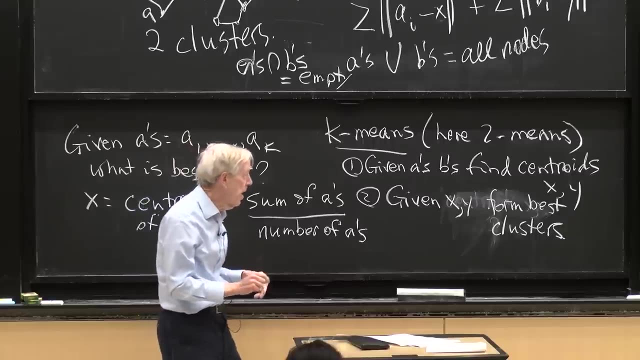 And then they're probably different from my original start. So now I've got new. Now I repeat step one. But let's just think: how do I form the best clusters? Well, I take a point And I have to decide: does it go with X? 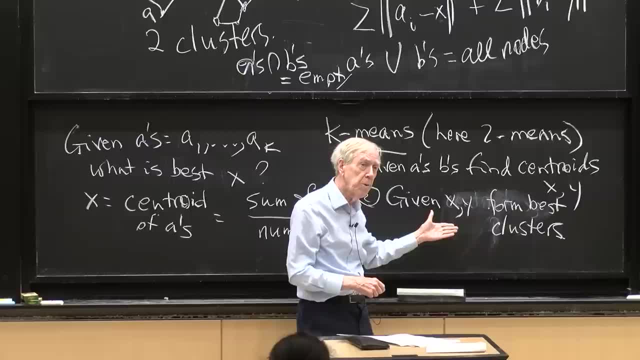 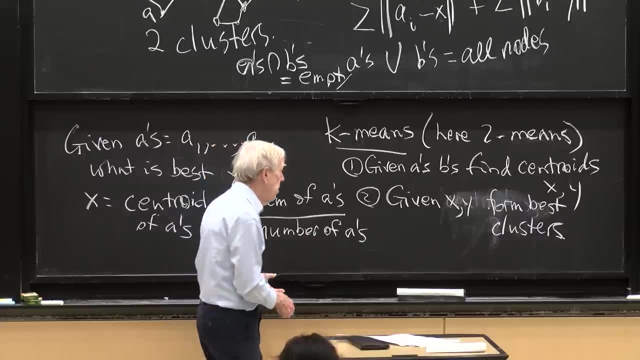 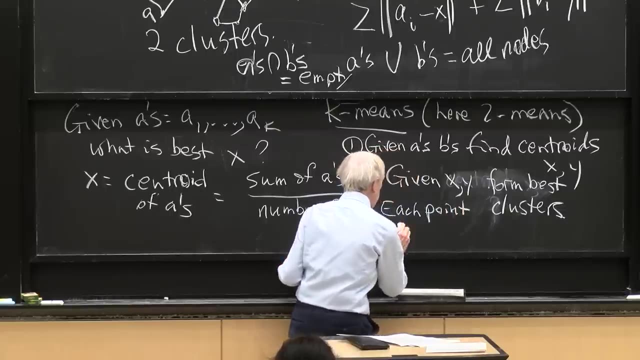 Or does it go in the X cluster, Or does it go in the cluster around Y? So how do I decide that, Just whichever one I choose, OK, OK, OK, OK, Which one it's closer to. So each point goes with each node. 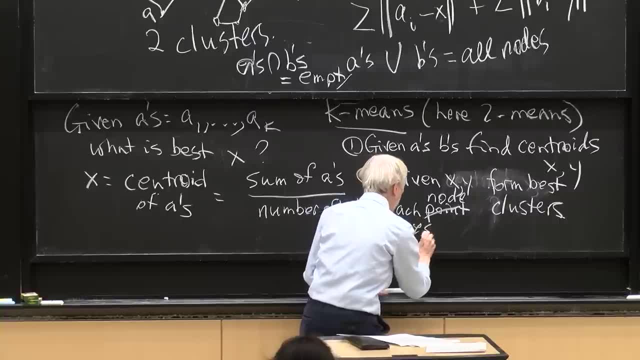 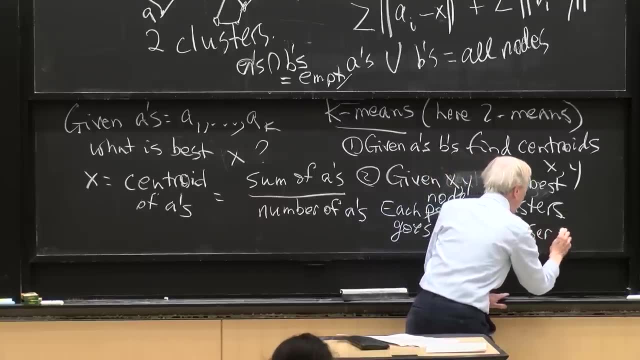 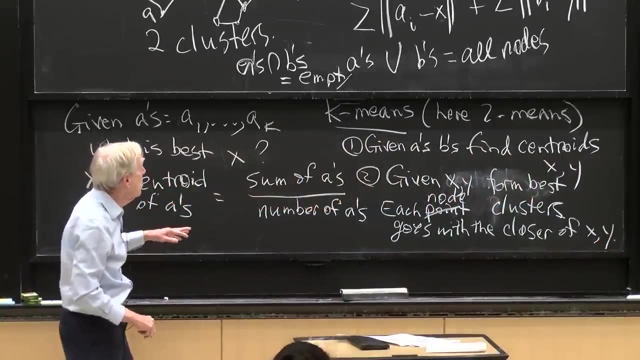 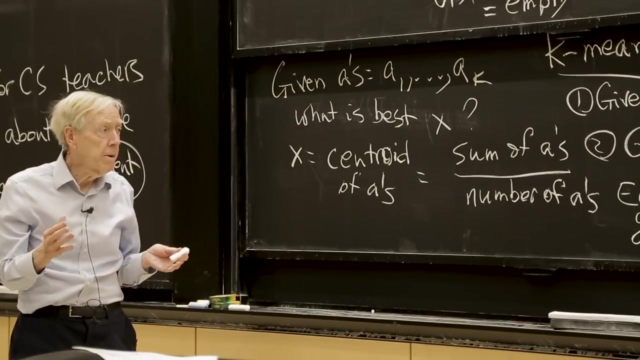 I could say each node goes with the closer of X and Y. So points that should have been So, points that should have been that are closer to X, now we're going to put them in the cluster around X, And does that solve the problem? 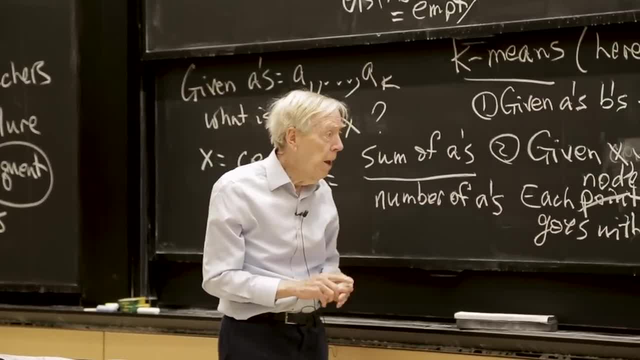 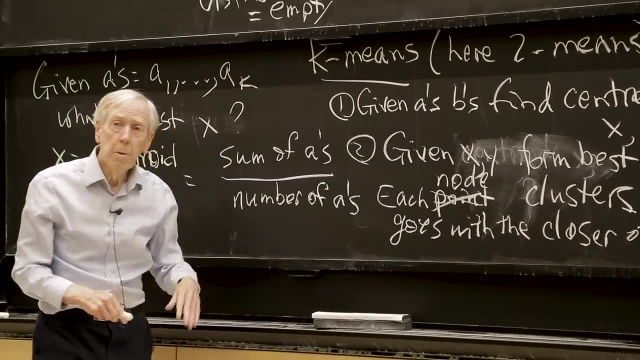 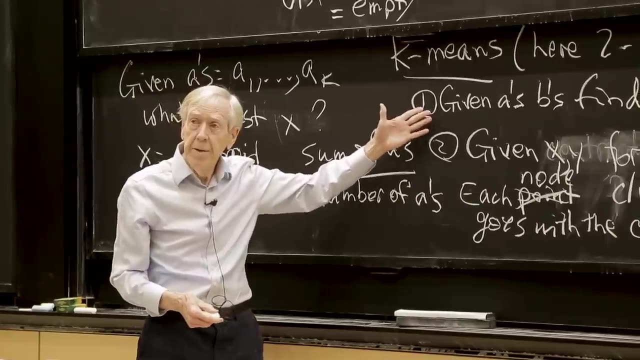 No, because well, it might, but it might not. We have to come back to step one. We've now changed the clusters. They'll have different centroids. So we repeat step one: find the centroids for the two new clusters. 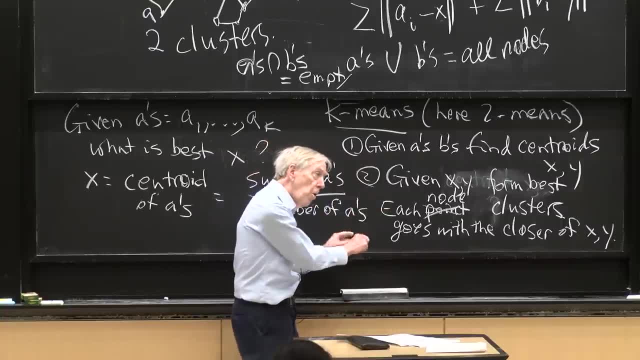 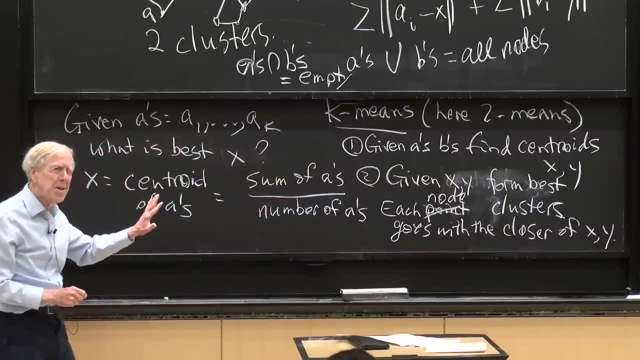 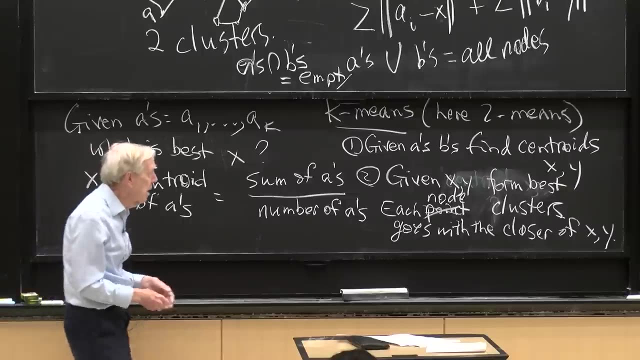 Then we come to step two, find the ones that should go with the two centroids, and back and forth. I don't know. I don't think there's a nice theory of convergence or rate of convergence, all the questions that this course is always asking. 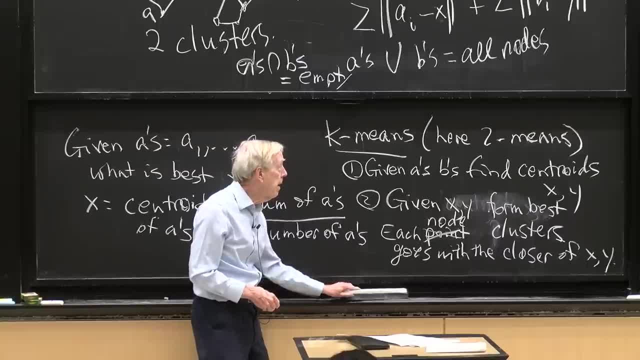 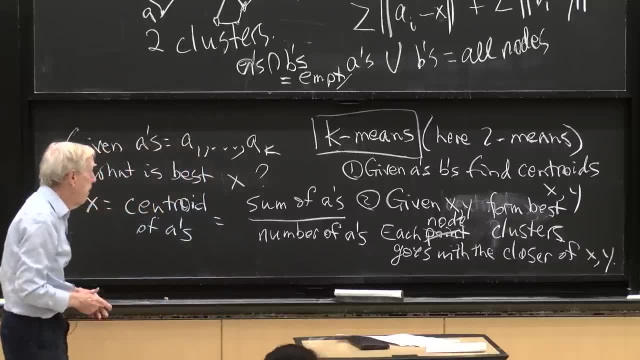 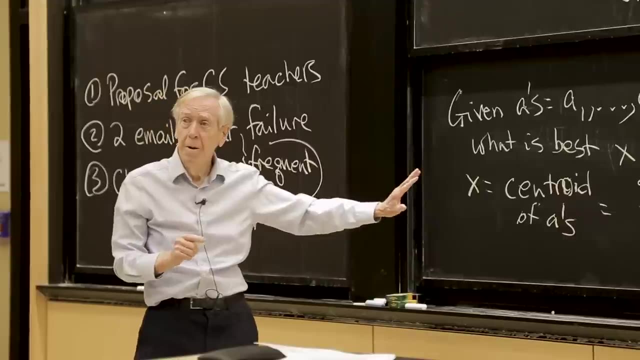 But it's a very popular algorithm. K means K would be to have K clusters. OK, OK, OK, So that's a. I'm not going to discuss the. I'd rather discuss some other ways to do this, to solve this problem. 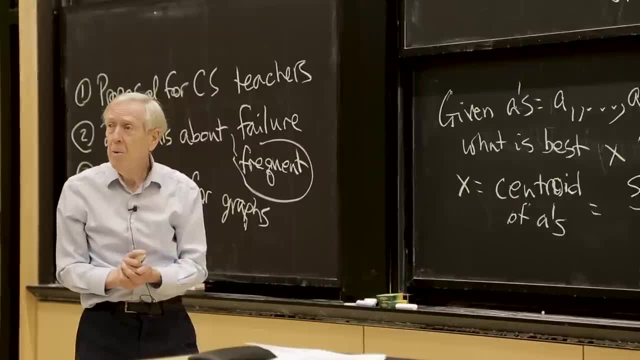 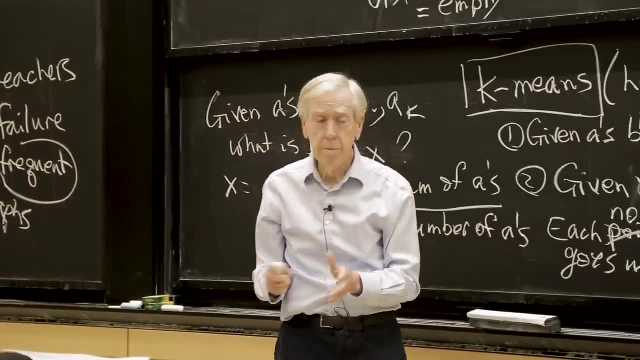 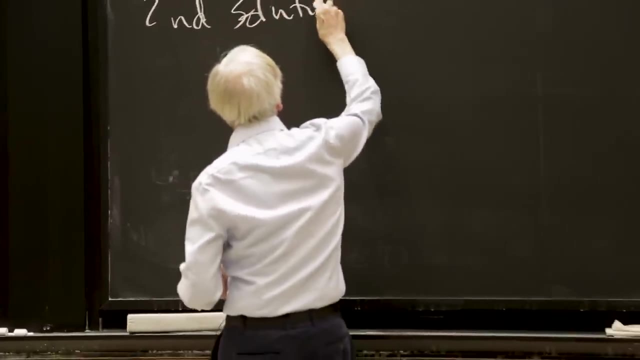 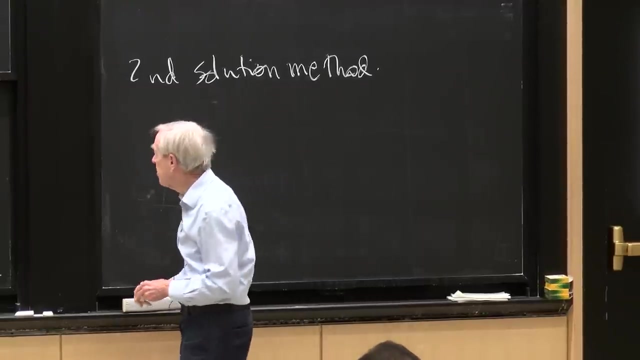 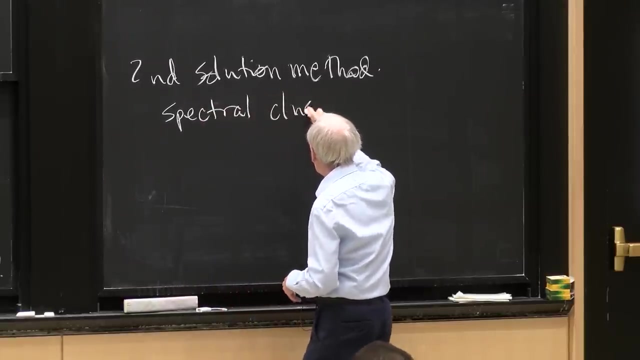 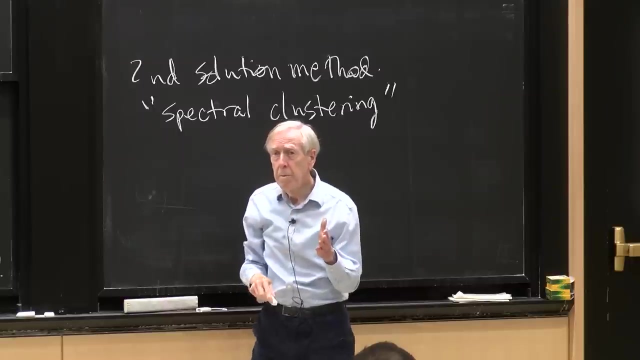 But that's one sort of hack that works quite well. OK, so second approach is what is coming next. Second solution method, And it's called the spectral clustering. That's the name of the method. And before I write down what you do, 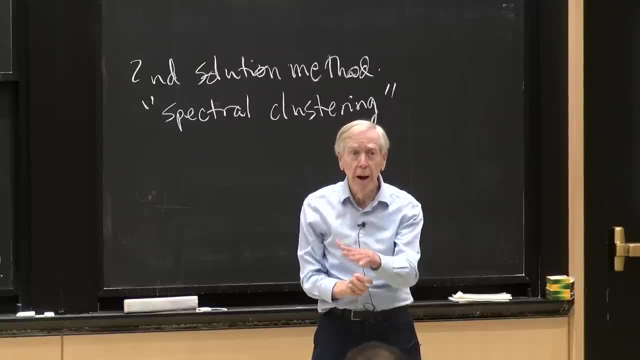 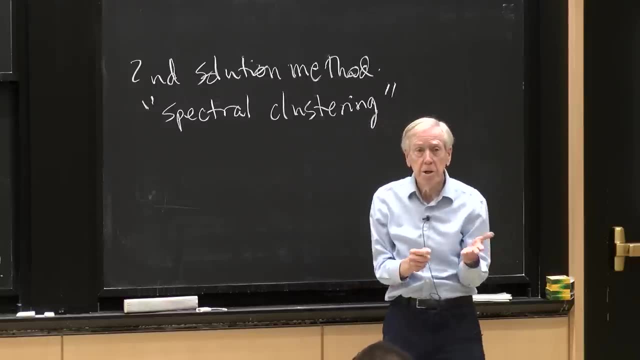 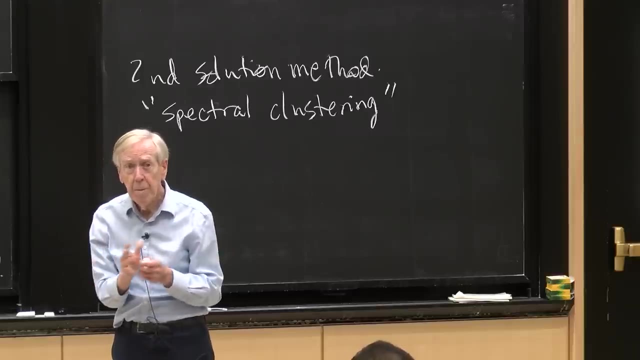 what does the word spectral mean? You see spectral graph theory, spectral clustering And in other parts of mathematics you see that word. You see spectral theorem. I gave you the most and I described it as the most important perhaps theorem in linear algebra. 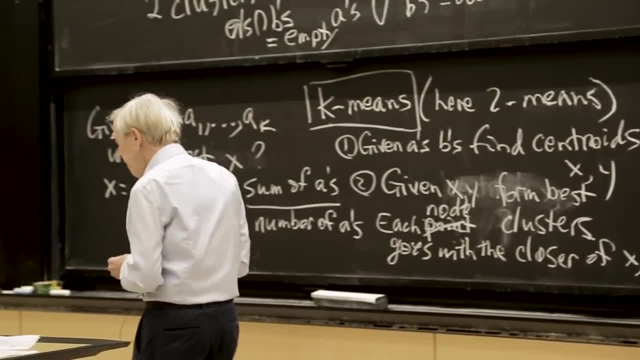 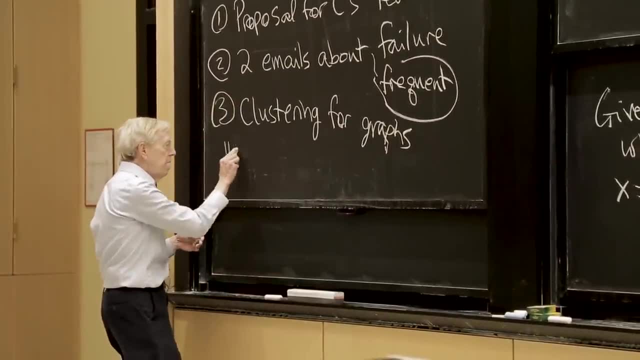 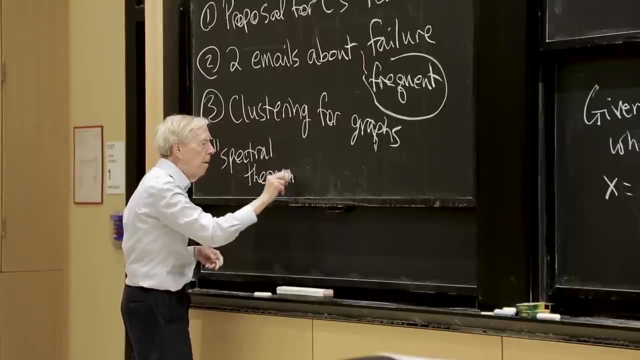 At least one of the top three is, so I'll write it over here, because it's not. it doesn't? this is a. it's the same word: spectral. Well, let me ask the question Again: what's that word spectral about? 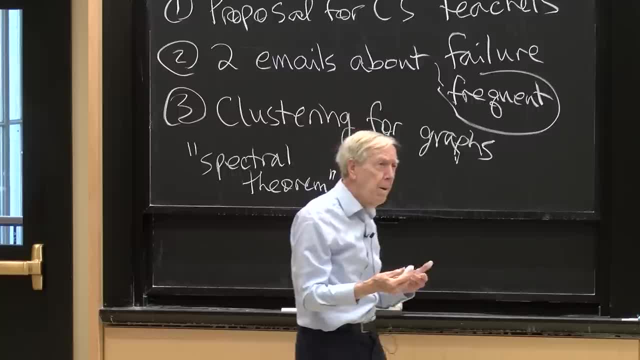 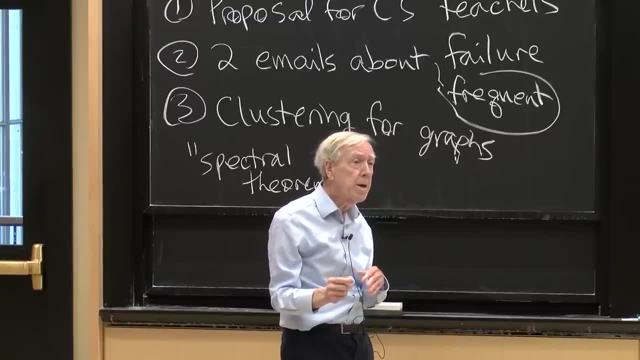 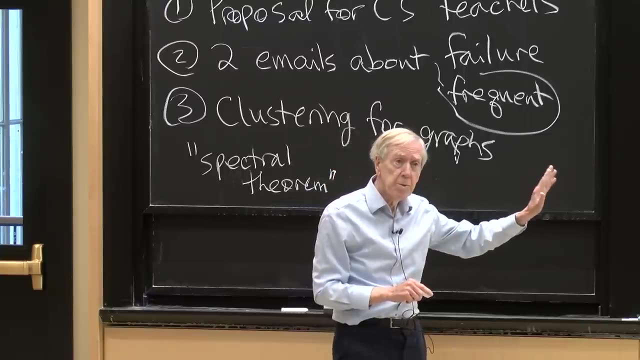 What does that mean? That means that if I have a matrix and I want to talk about its spectrum, what is the spectrum of the matrix? It is the eigenvalues. So spectral theory, spectral clustering, is using the eigenvalues of some matrix. 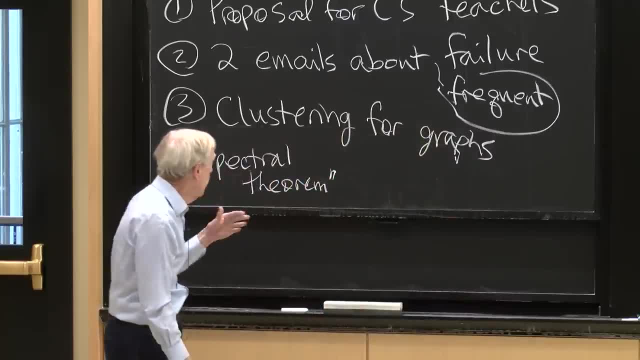 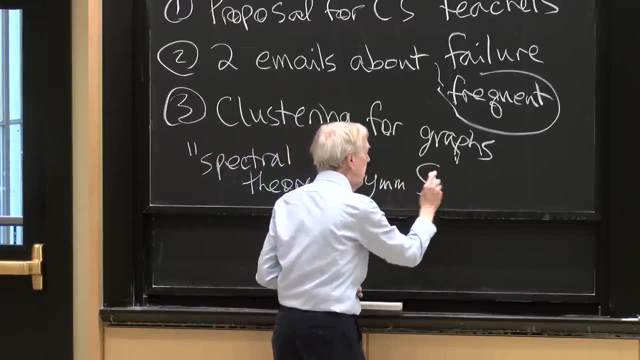 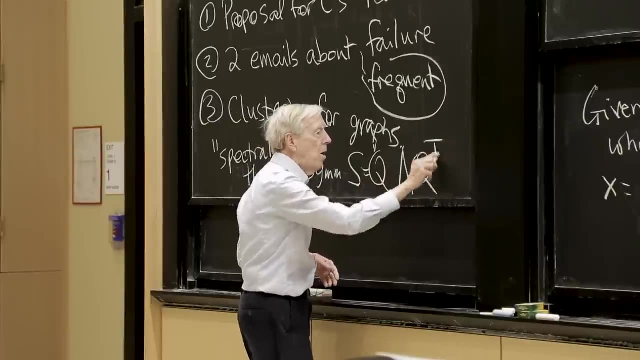 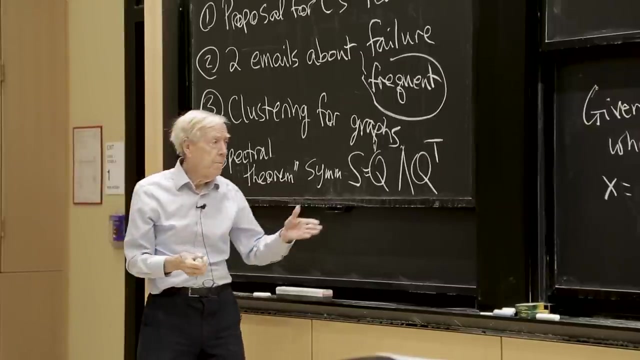 That's what that spectral is telling me. Yeah, So there's spectral theory. Spectral theorem, of course, is that for a symmetric matrix S, the eigenvalues are real and the eigenvectors are orthogonal. And don't forget what the real full statement is here. 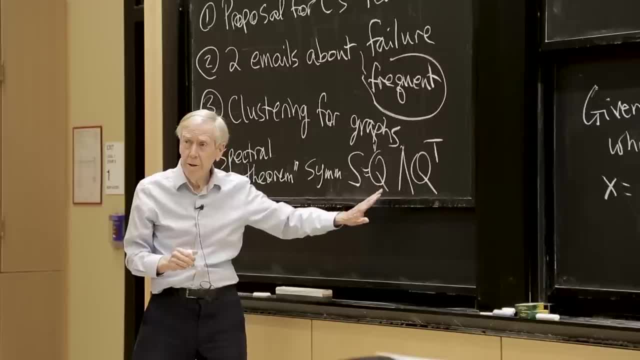 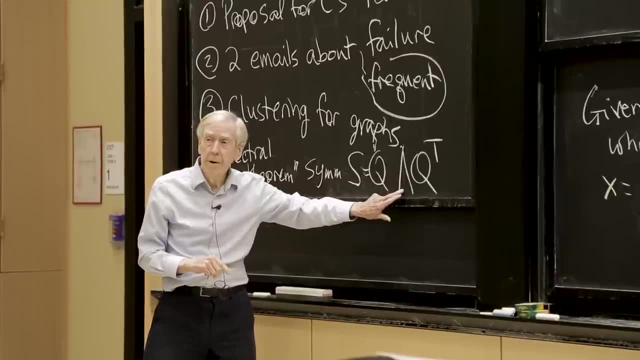 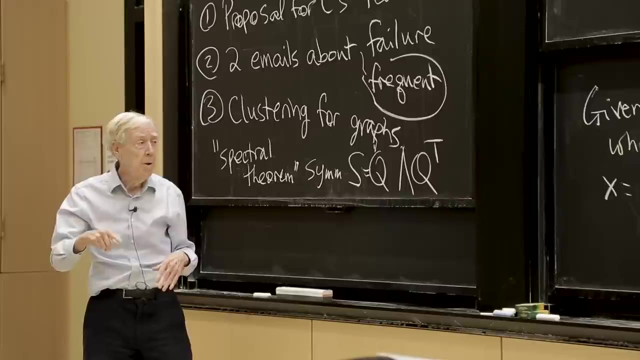 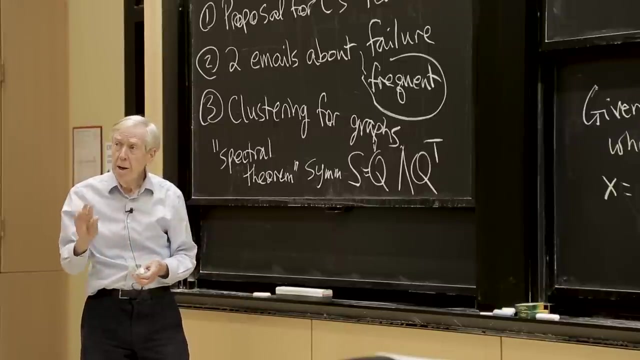 because there could be repeated real eigenvalues. And what does the spectral, The spectral theorem, tell me for symmetric matrices? if that, if lambda equals 5, is repeated four times, if it's a four times solution of the equation that gives eigenvalues, then what's the conclusion? 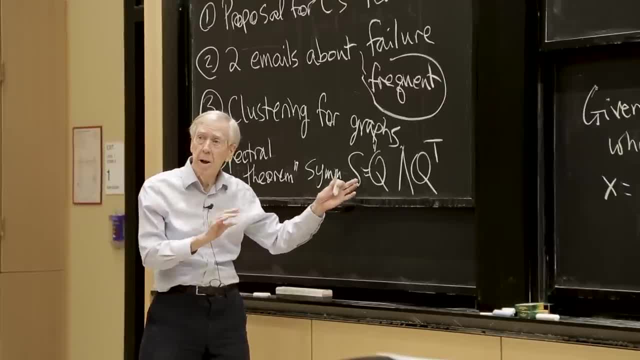 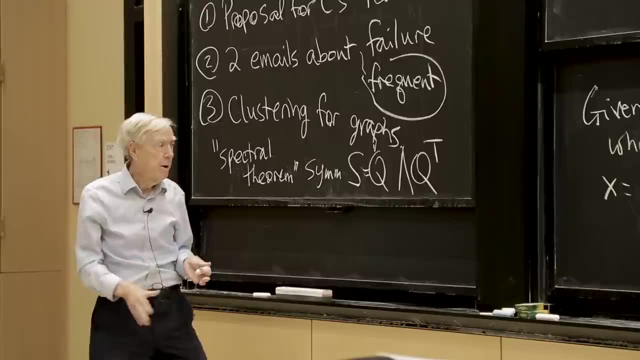 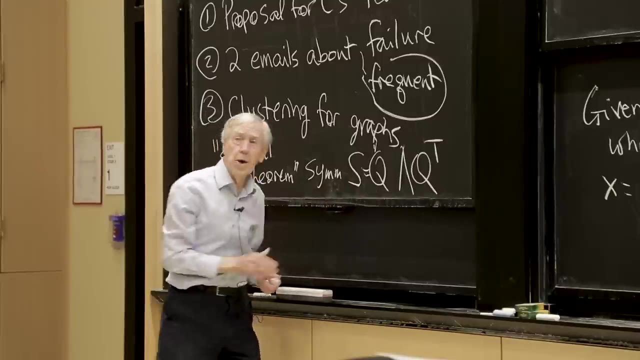 Then there are four independent orthogonal eigenvectors to go with it. We can't say that about matrices, We can't say that about all matrices, But we can say it about all symmetric matrices And in fact those eigenvectors are orthogonal. 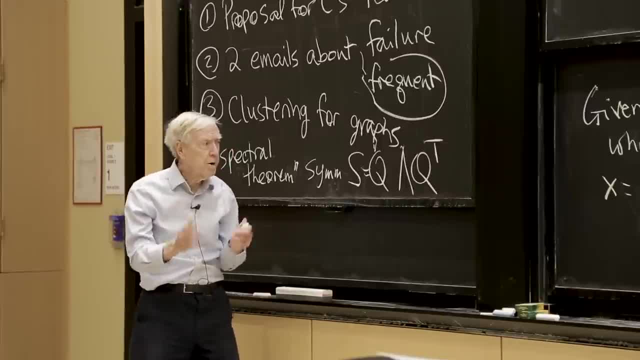 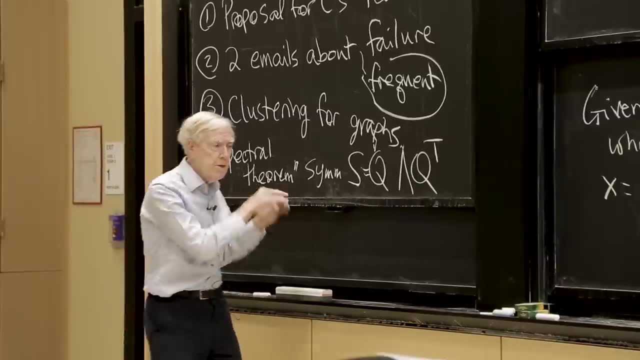 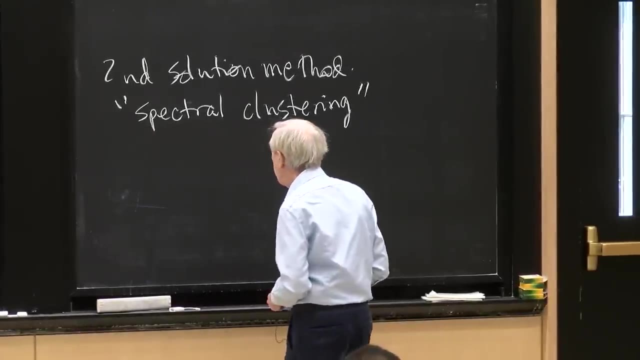 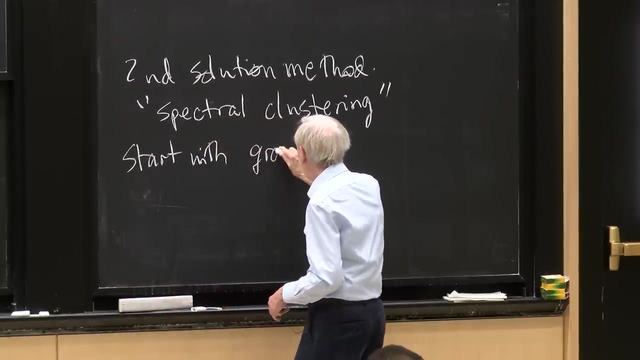 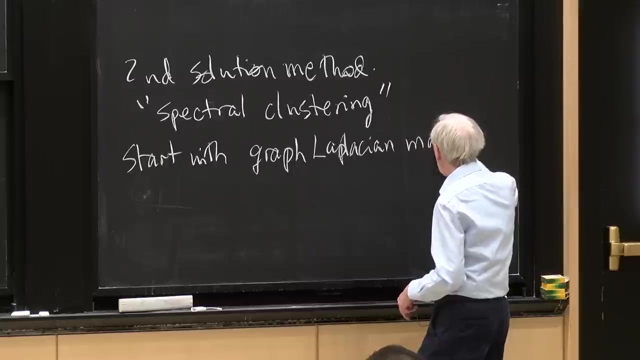 So we're even saying more. We can find four orthogonal eigenvectors that go with a multiplicity for eigenvalue. OK, that's spectral theorem. Spectral clustering starts with the with the graph Laplacian matrix. May I remember what that matrix is? 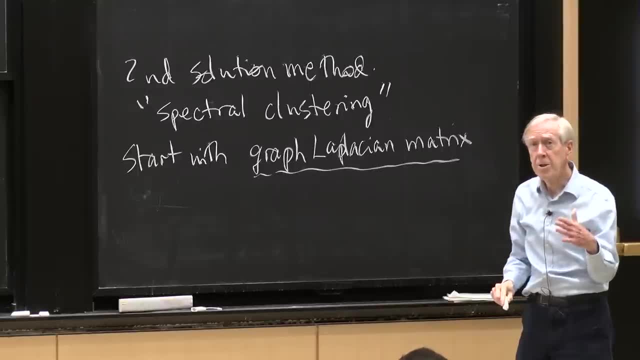 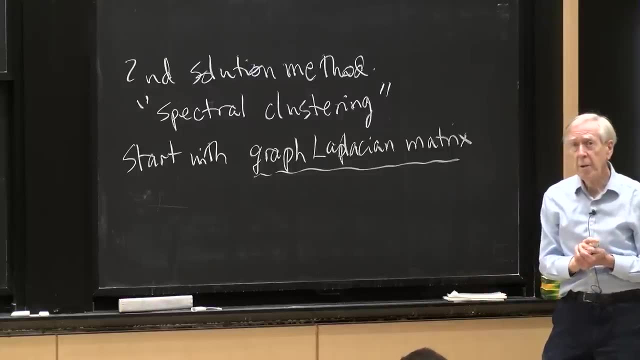 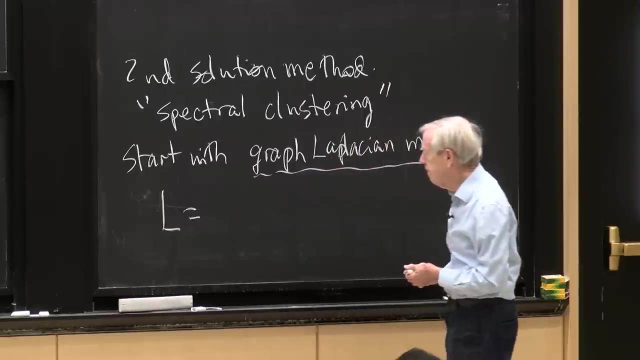 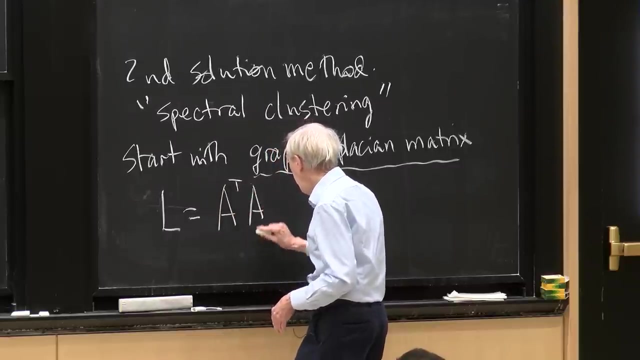 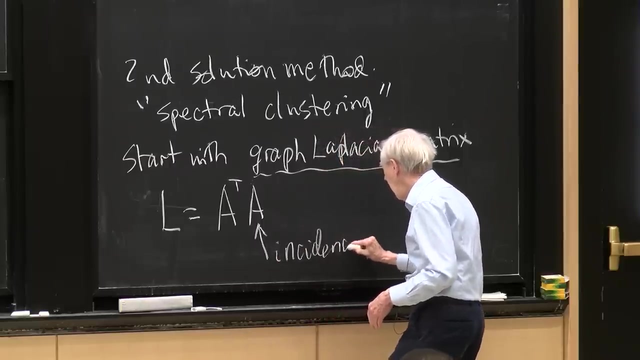 Because that's the key connection of linear algebra to graph theory- is the properties of this graph, Laplacian matrix. OK, so let me say L for Laplacian, So that matrix. one way to describe it is as A transpose A, where A is the incidence matrix. 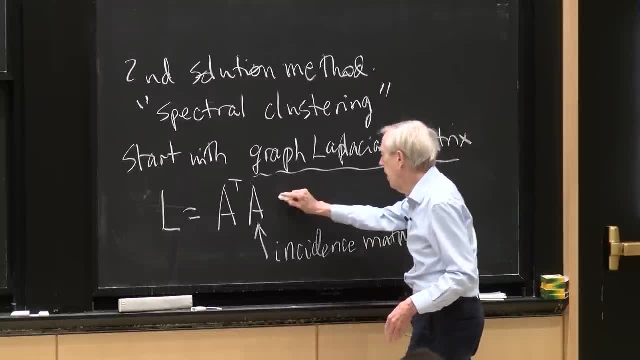 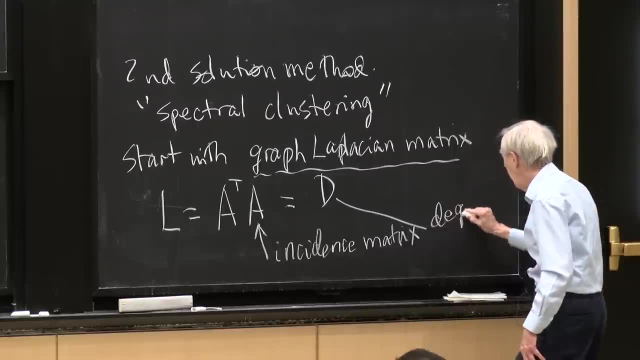 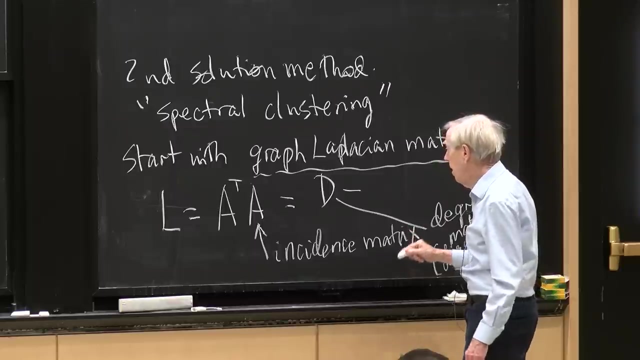 of the graph, Or another way we'll see: is the D the degree matrix? That's the degree matrix, OK, OK, OK, OK, Diagonal, And I'll do an example just to remind you: Minus the- well, I don't know what I've called this one. 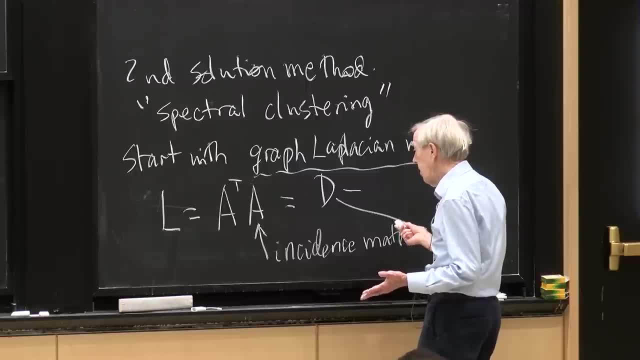 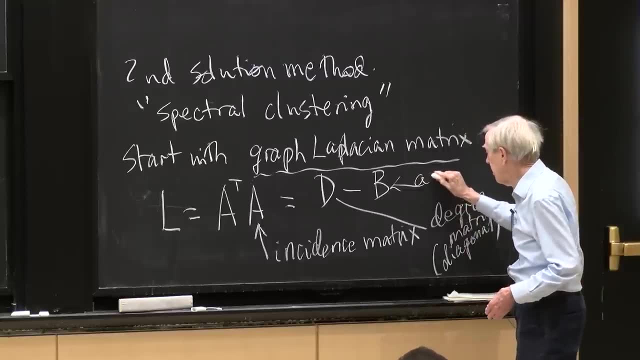 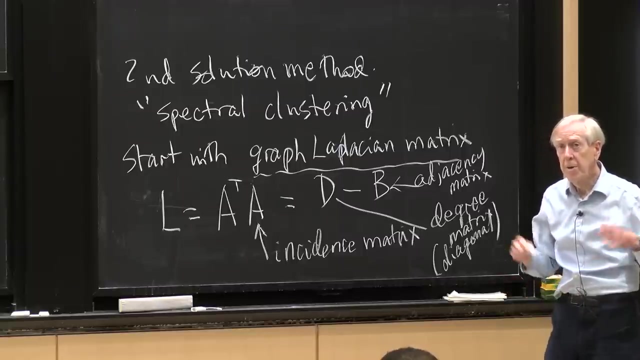 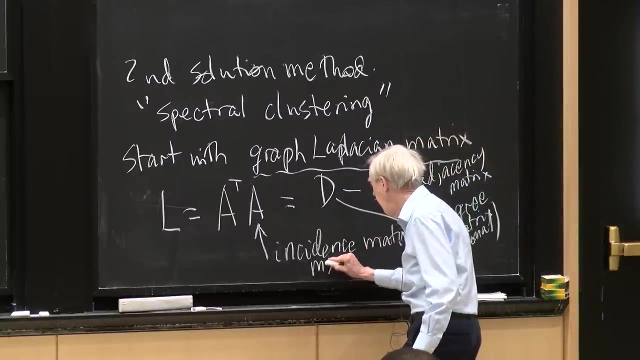 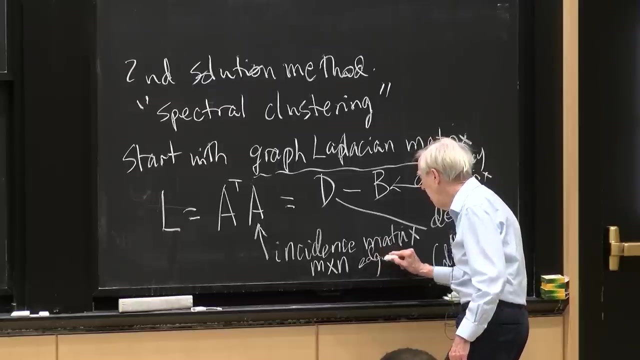 Uh, shall I call it B for the moment? And what matrix is B? That's the adjacency matrix. So really you should know these four matrices. They're the key four matrices associated with any graph. The incidence matrix, that's m by n, edges and nodes, edges. 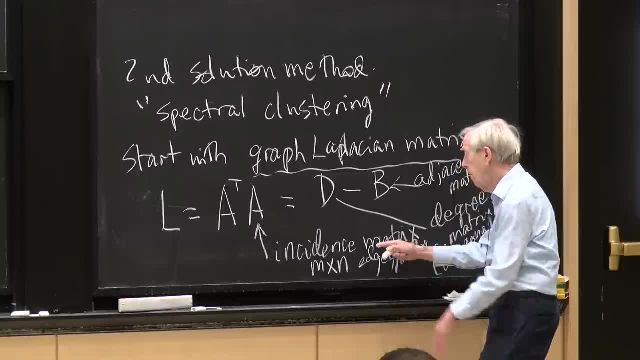 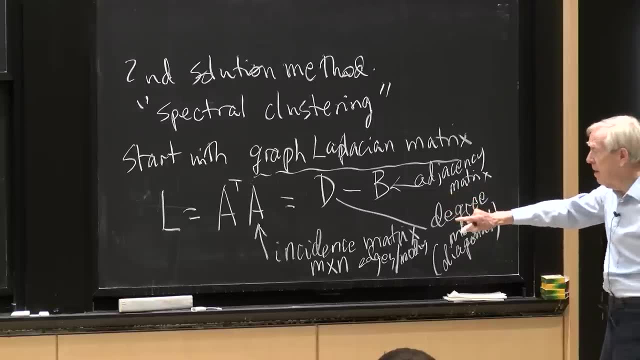 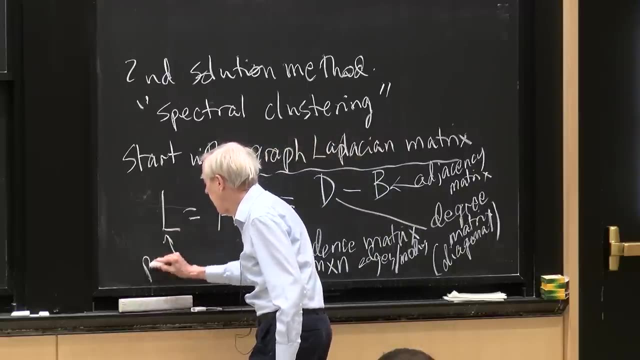 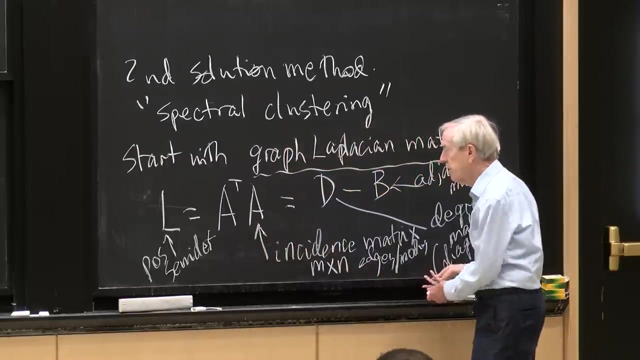 and nodes, So it's rectangular. but I'm forming A transpose A here, So I'm forming a symmetric, positive, semi-definite matrix. So this little Poisson is symmetric, positive, semi-definite. Yeah, let me just recall what all these matrices 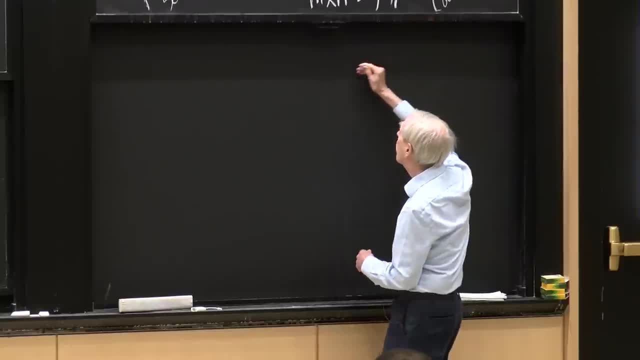 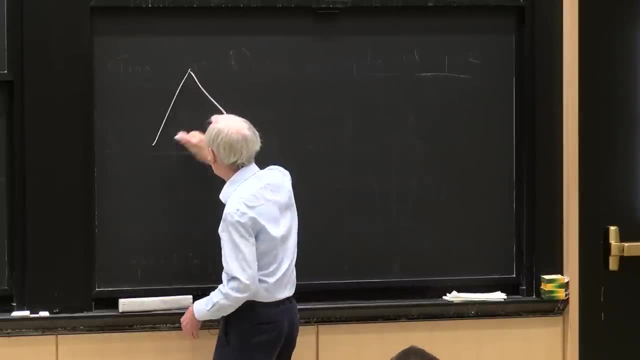 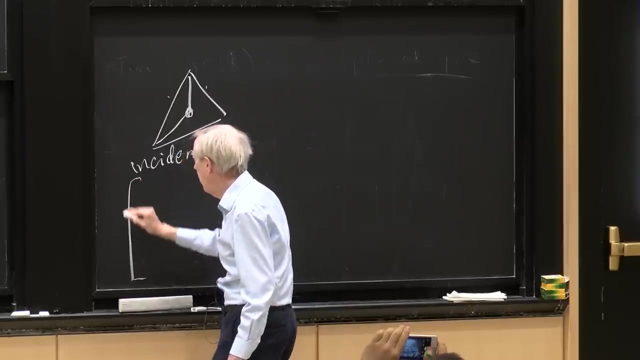 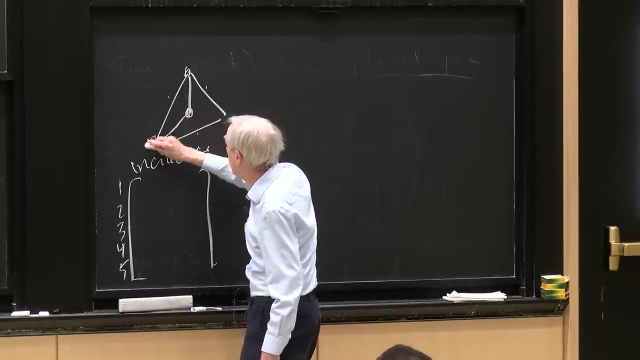 are for a simple graph. OK, so I'll just draw a graph. OK, so the incidence matrix: there are 1,, 2,, 3,, 4,, 5 edges, so five rows. There are four nodes: 1,, 2,, 3, and 4,, so four columns. 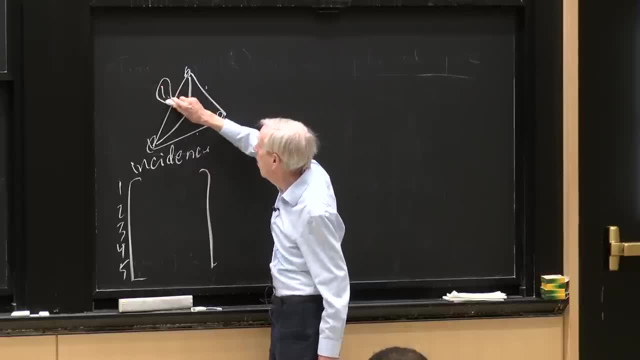 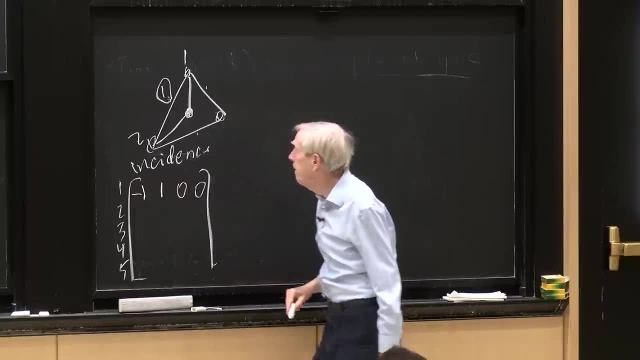 And a typical row. It would be edge 1, going from node 1 to node 2.. So it would have a minus 1 and a 1 there, And let me take edge 2, going from 1 to node 3.. 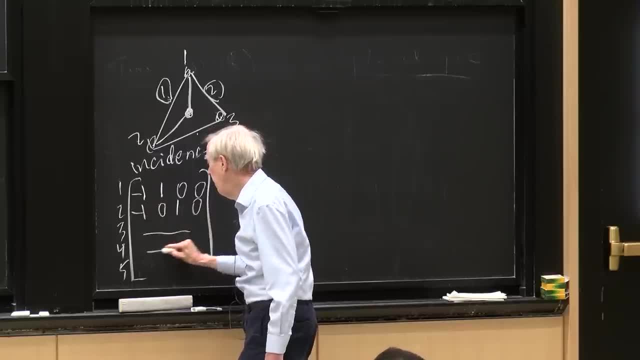 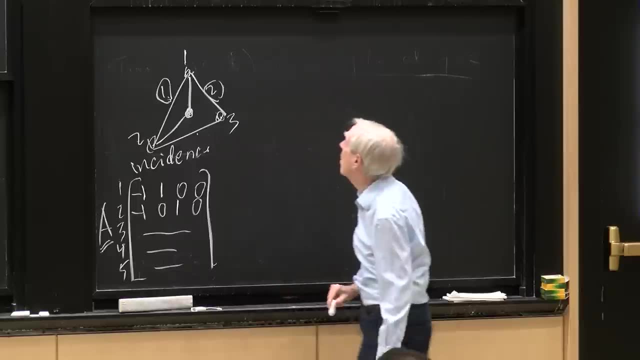 So it would have a minus 1 and a 1 there, so on. So that's the incidence matrix, A. OK, what's the degree matrix? That's simple, The degree matrix. Well, A transpose A. this is n by n. 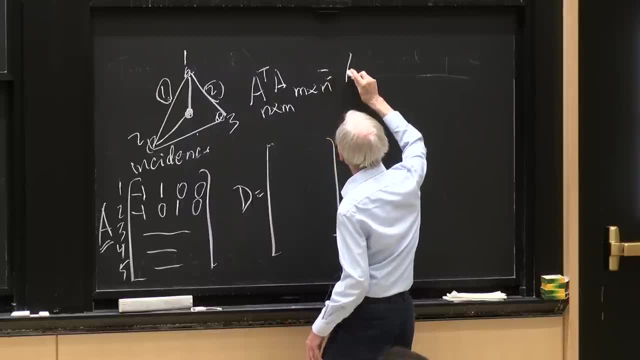 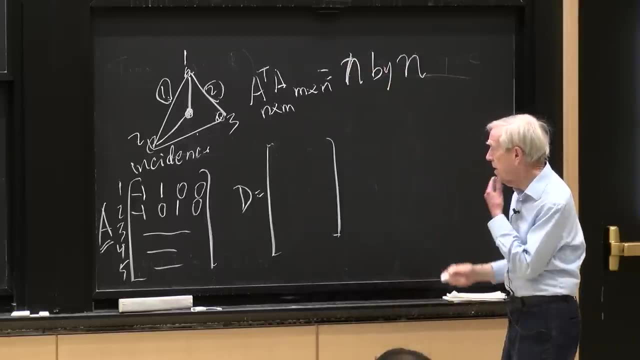 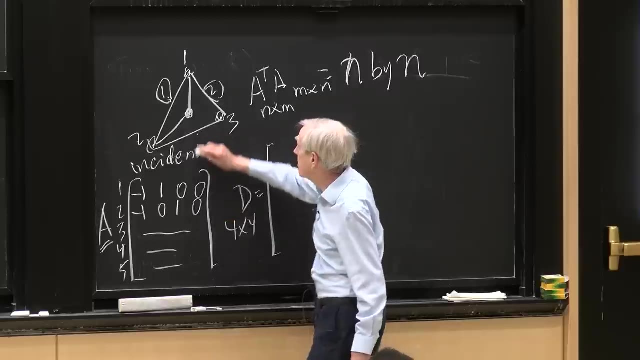 This is n by m, So it's n by n. OK, in this case 4 by 4.. So the degree matrix will be 4 by 4, n by n, And it will tell us the degree of that, which means: 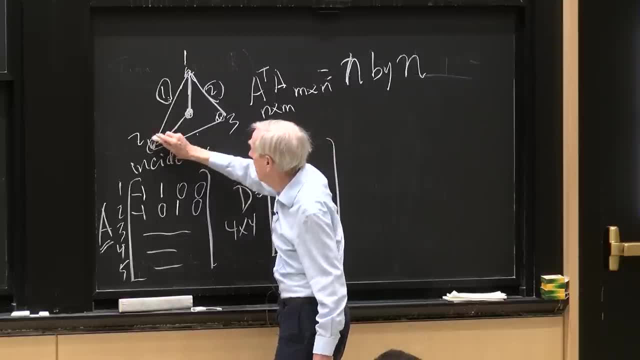 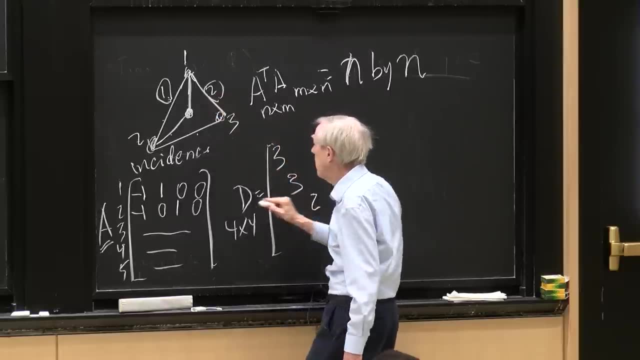 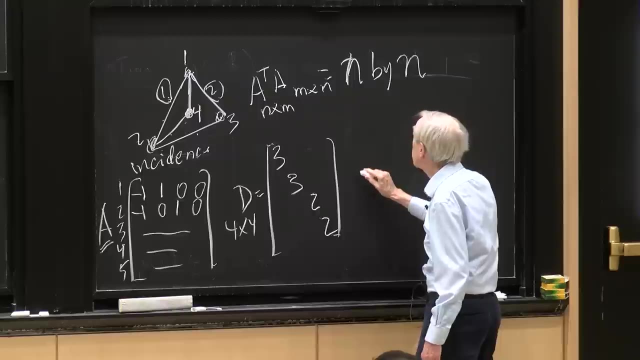 which we just count the edges. So it's three edges going in Node 2, three edges going in. Node 3 has just two edges And node 4 has just two edges. So that's the degree matrix And then the adjacency matrix that I've called B. 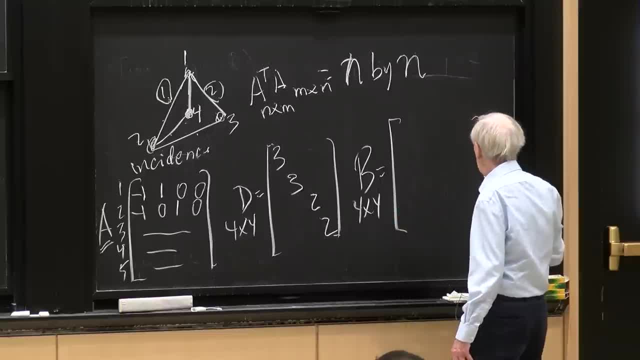 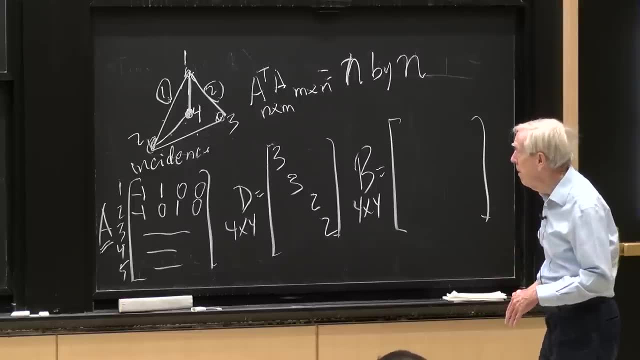 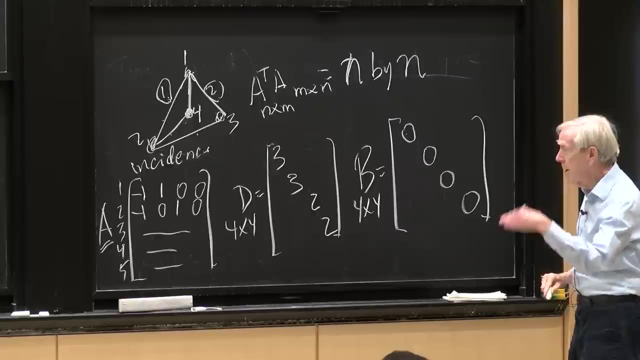 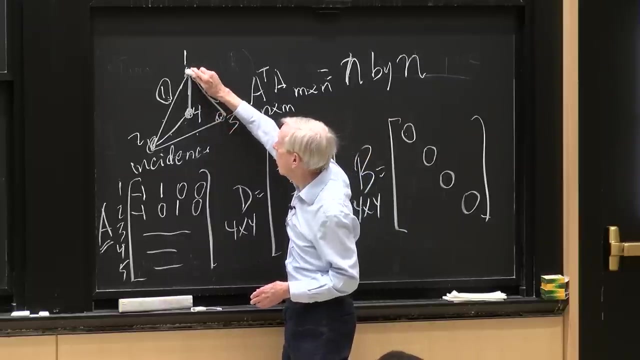 is also 4 by 4.. And what is it? It tells us which node is connected to which node. So I don't allow nodes edges that connect a node to itself. So 0 is on the diagonal. So which nodes are connected to node 1?? 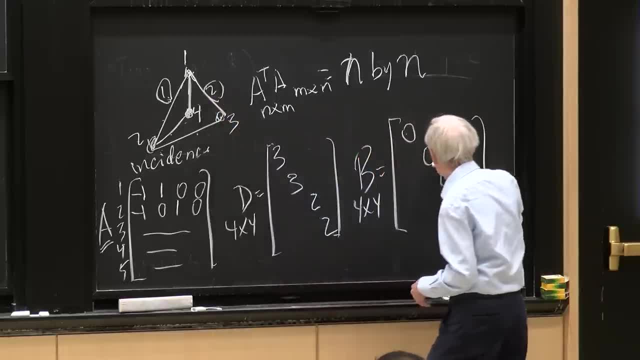 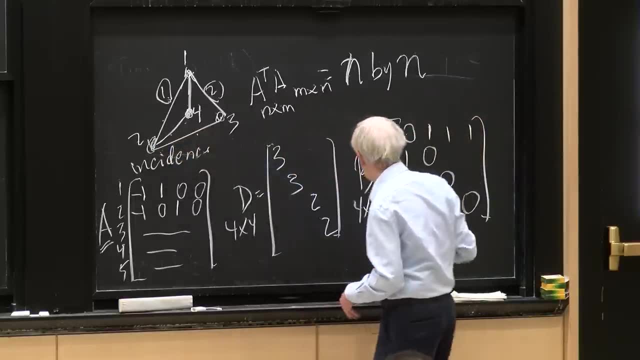 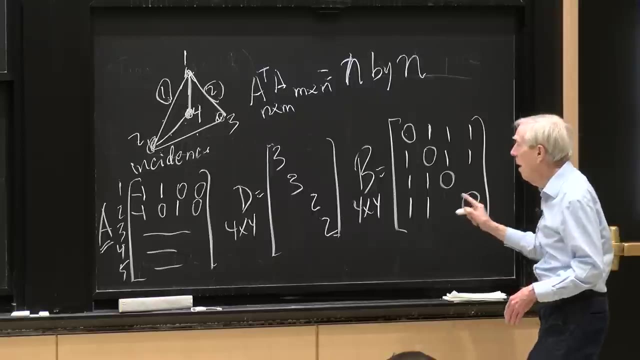 Well, all of 2 and 4 and 3 are connected to 1.. So I have 1's there. Node 2, all three nodes are connected to node 2.. So I'll have the second column and row. We'll have all three 1's. 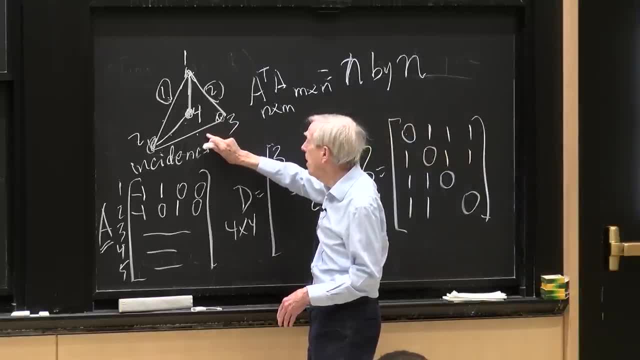 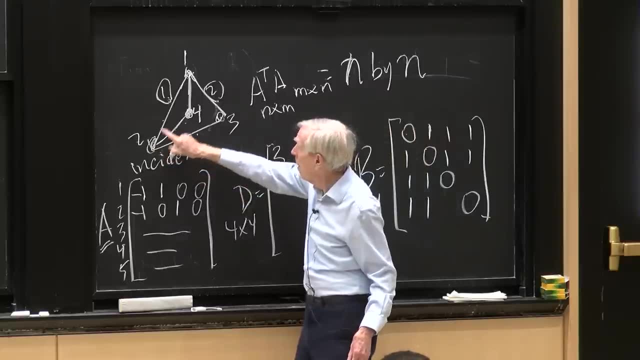 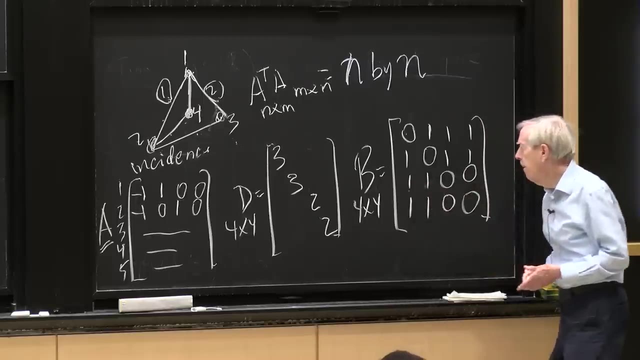 How about node 3?? OK, only edges. only two edges are connected, Only two nodes are connected to 3.. 1 and 2, but not 4.. So 1 and 2 I have, but not 4.. 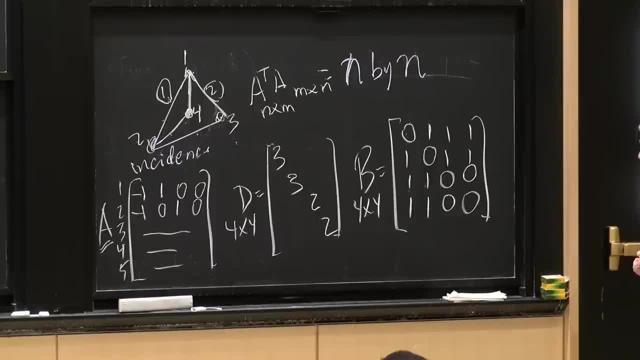 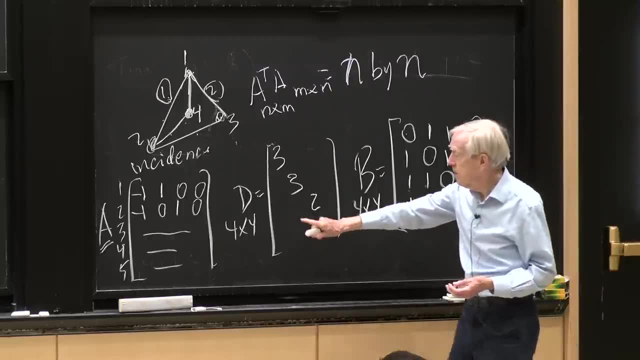 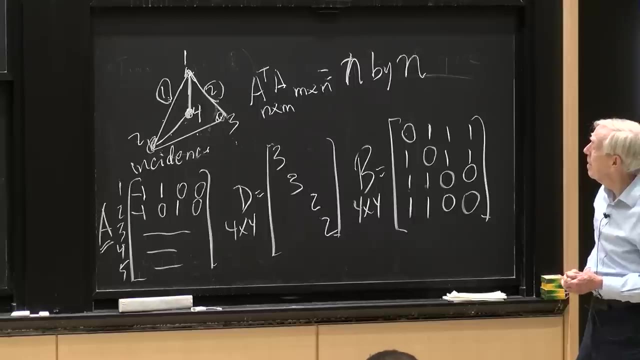 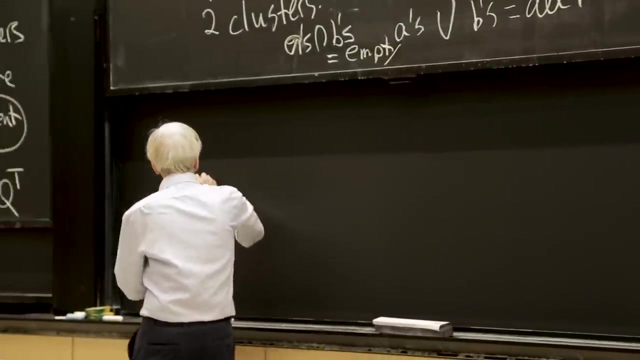 OK, so that's the adjacency matrix. Is that right? Think so. This is the degree matrix, This is the incidence matrix And that formula gives me the Laplacian. OK, let's write down the Laplacian. So, if I use the degree minus B, that's easy. 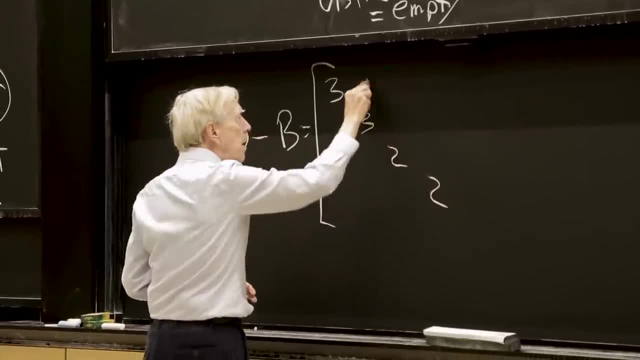 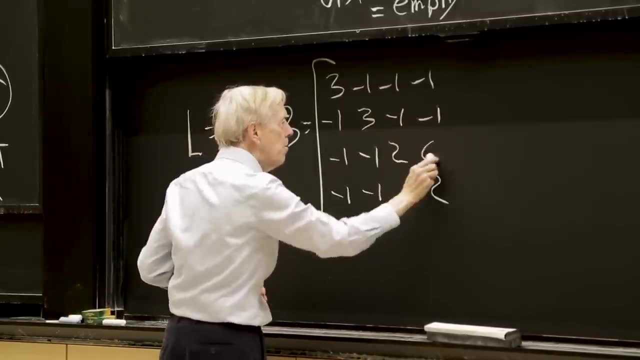 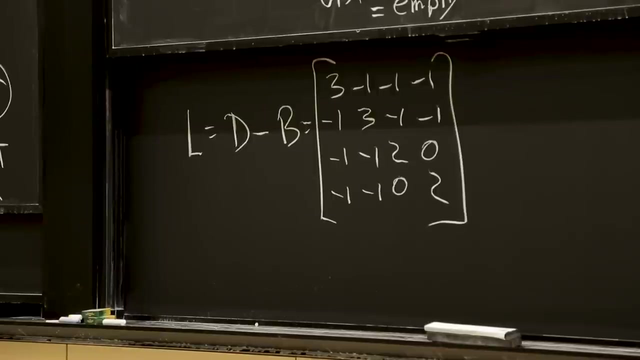 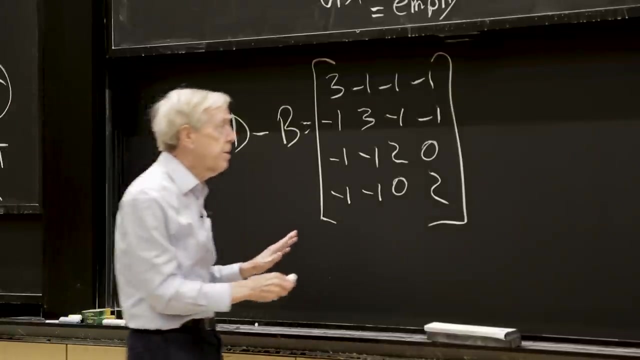 The degrees were 3, 3,, 2, and 2.. Now I have these minuses And those were 0.. OK, So that's a positive semi-definite matrix. Is it a positive definite matrix? So let me ask: is it singular or is it not singular? 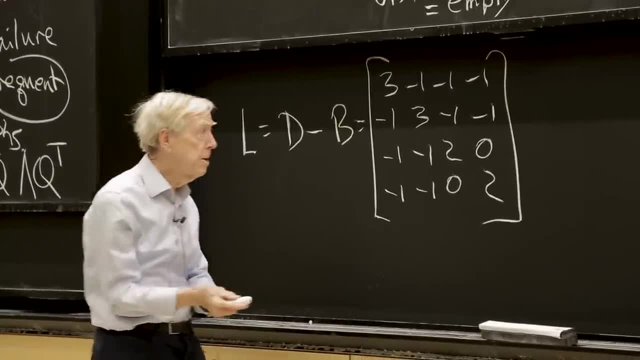 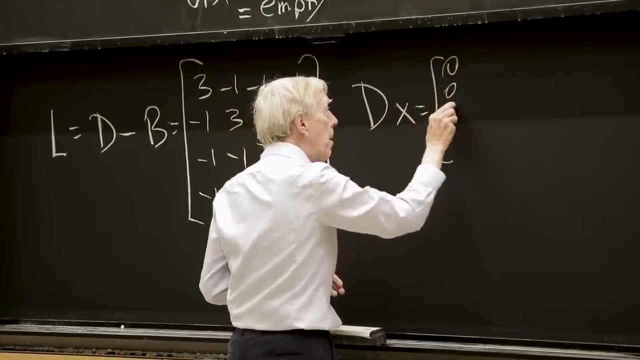 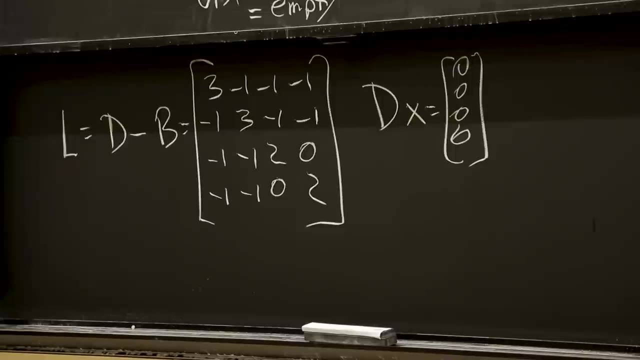 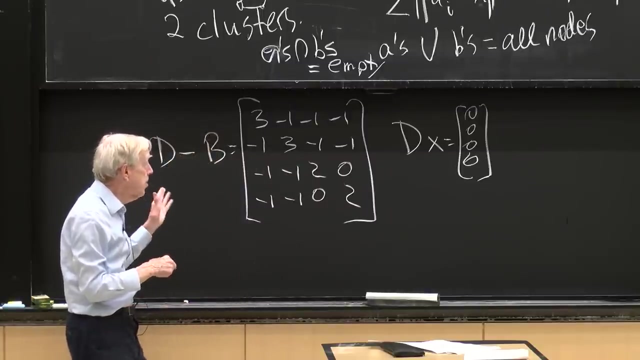 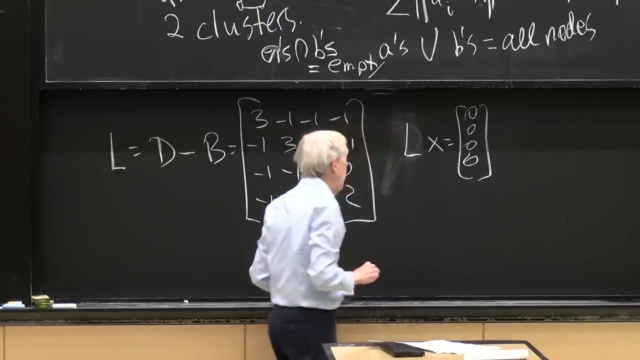 Is there a vector in its null space or is there not a vector in its null space? Can you solve? dx equals all 0's, And of course you can. Everybody sees that the vector of all 1's will be a solution to L. I'm sorry, I should be saying L here. 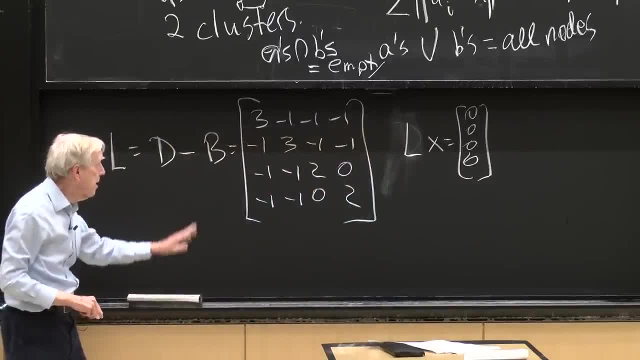 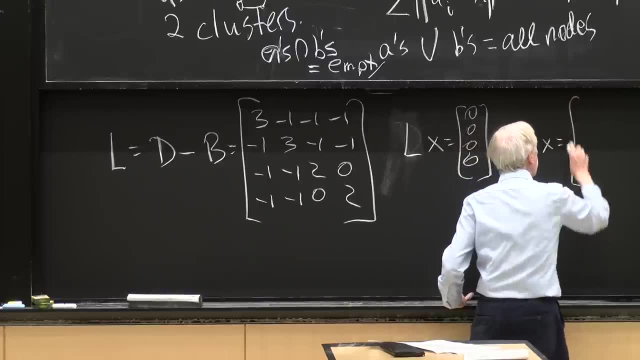 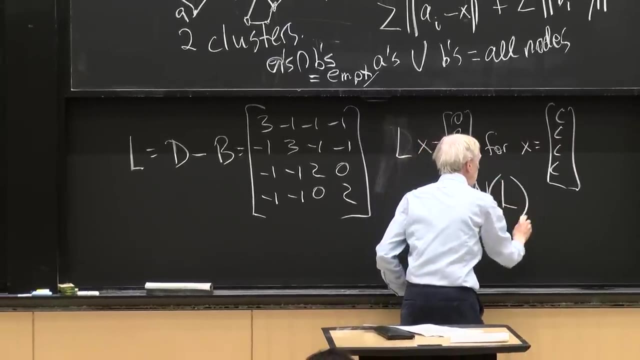 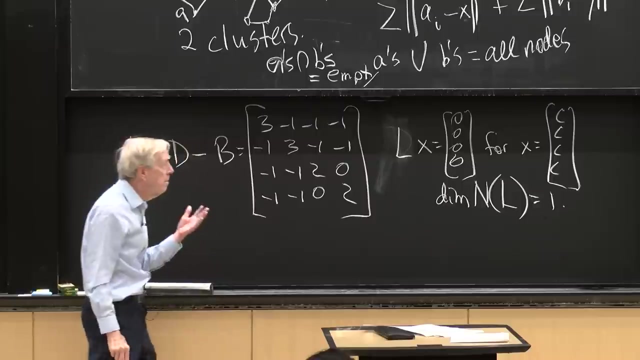 Lx equals 0.. Lx equals 0 is 4.. It's a whole line of a one-dimensional. The null space of L has dimension 1.. It's got one basis vector: 1,, 1,, 1,, 1.. 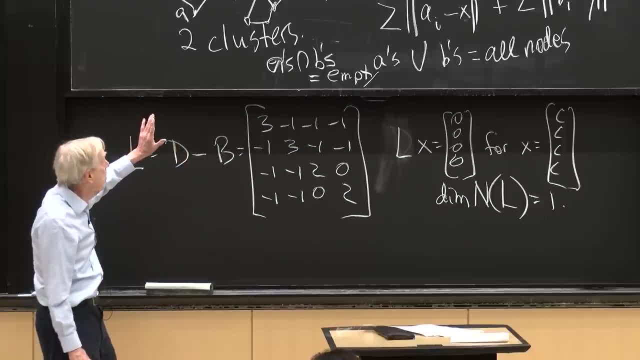 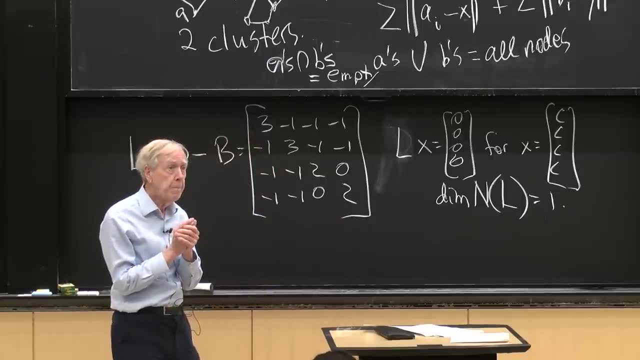 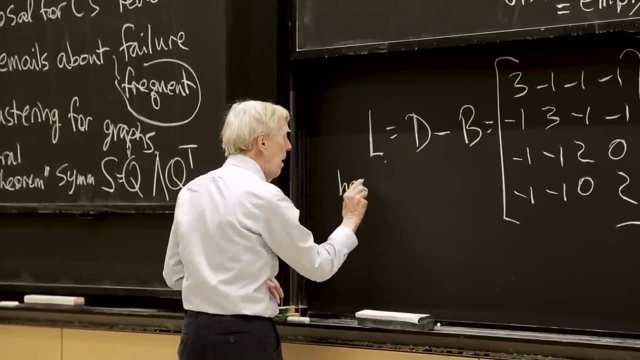 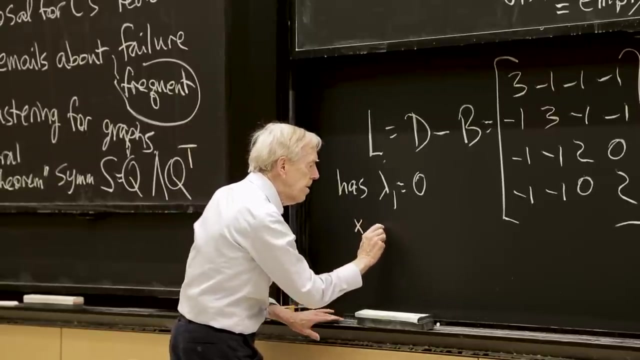 And that will always happen with the graph setup that I've created. OK, so that's the first fact That this positive semi-definite matrix L has lambda. 1 equals 0.. And the eigenvector is constants: c, c, c, c. 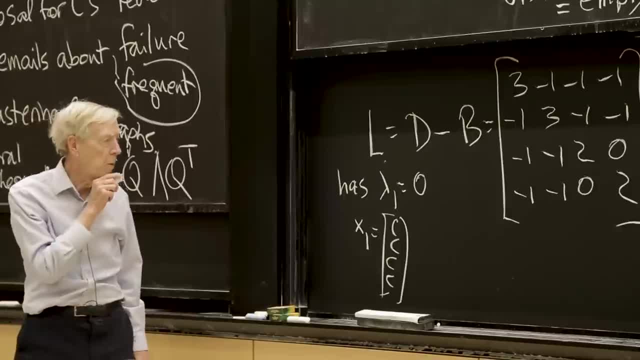 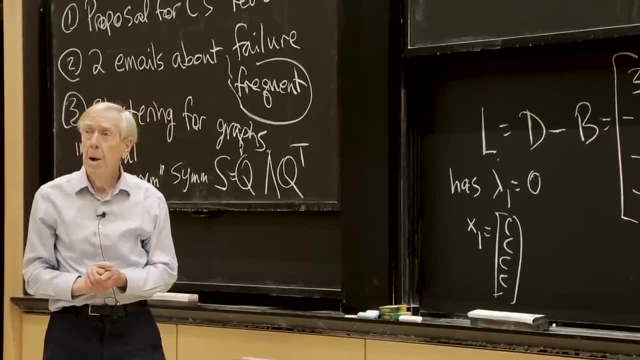 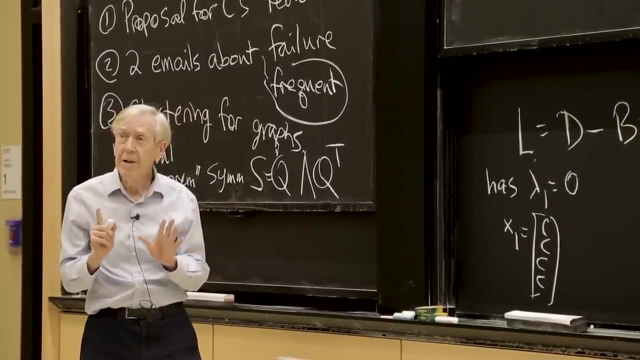 the one-dimensional eigenspace, Or 1,, 1,, 1, 1 is the typical eigenvector. OK, Now Back to graph clustering. The idea of graph clustering is to look at the Fiedler eigenvector. 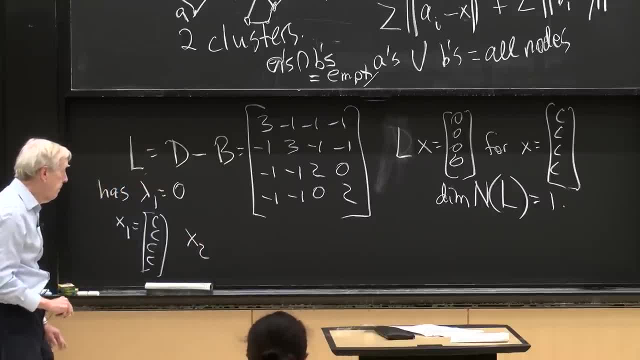 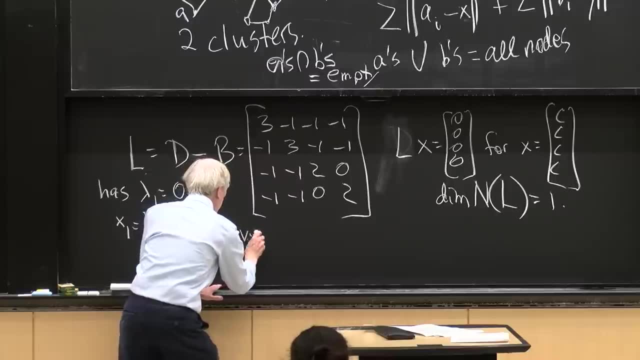 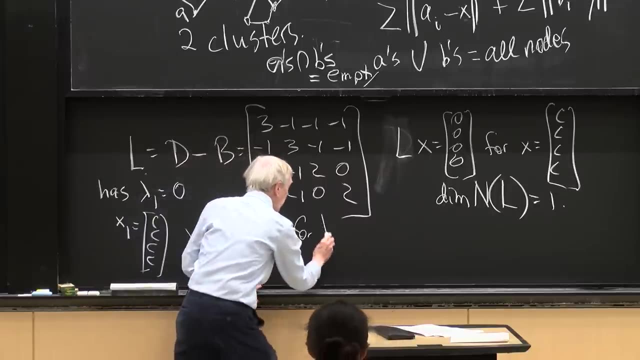 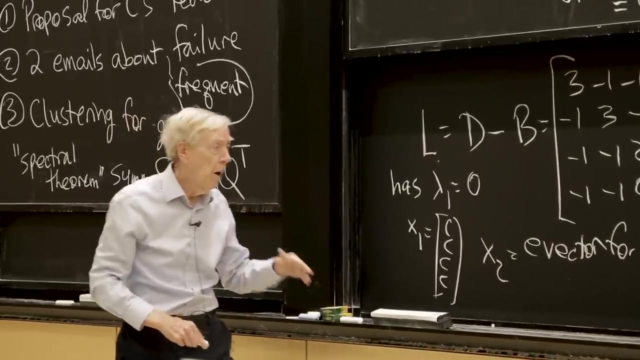 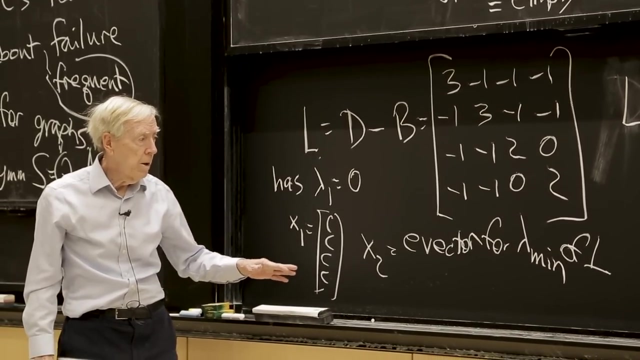 This is called x2, is the next eigenvector, is the eigenvector for the smallest positive eigenvalue for lambda min Excluding 0. So the smallest eigenvalue of L, the smallest eigenvalue and its eigenvector, this is called the Fiedler vector. 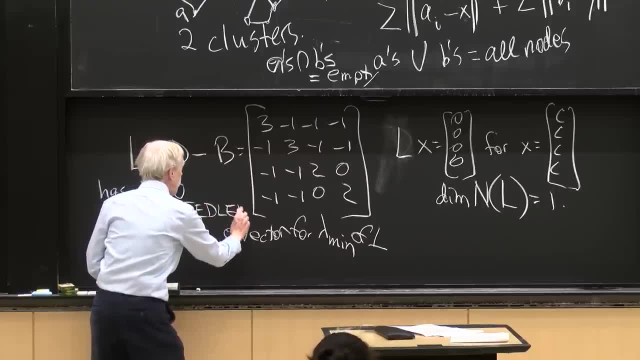 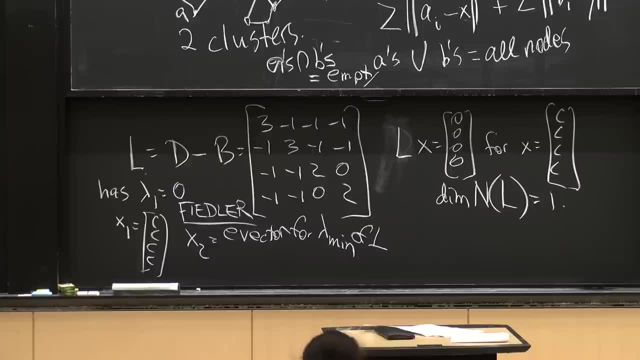 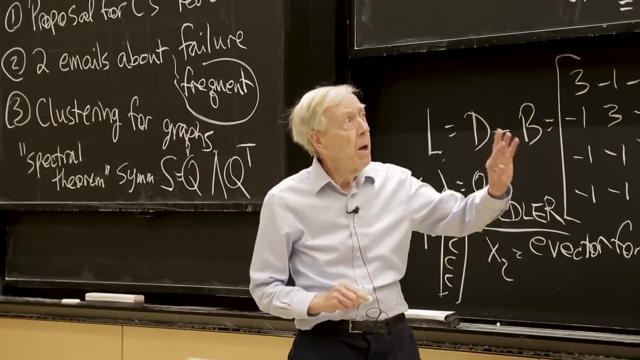 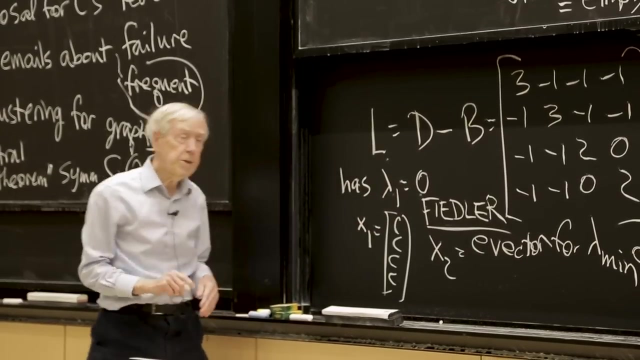 named after the Czech mathematician, a great man in linear algebra. OK OK, And he studied this vector, this situation. So everybody who knows about the graph Laplacian is aware that its first eigenvalue is 0 and that the next eigenvalue is important. 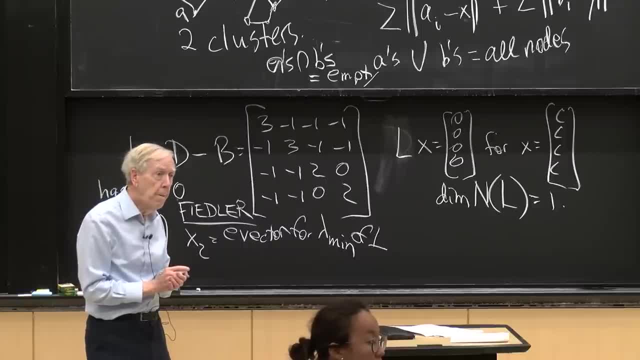 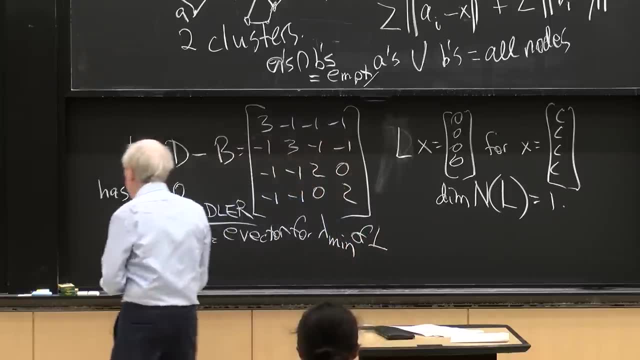 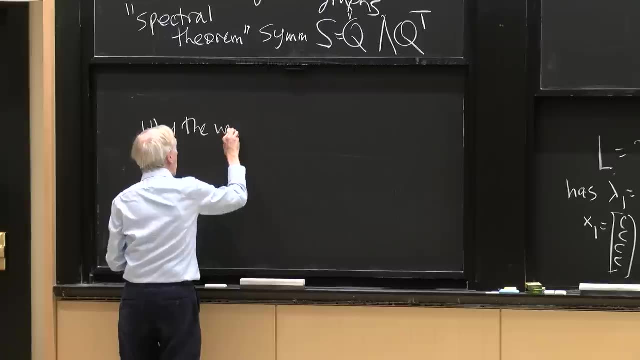 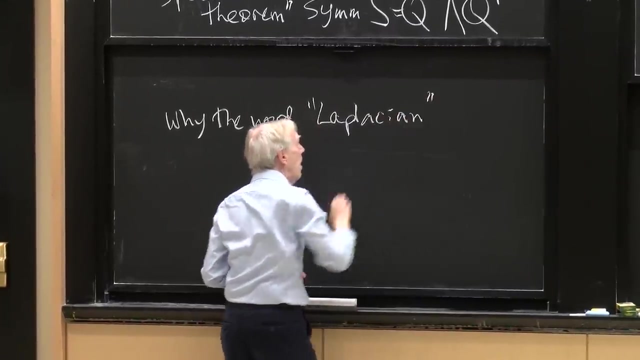 Yeah, Is the graph Laplacian named the Laplacian because it has connections To Laplace's equation? yes, Yeah, That's a good question. So why the word, the name, Laplacian? So, yeah, That's a good question. 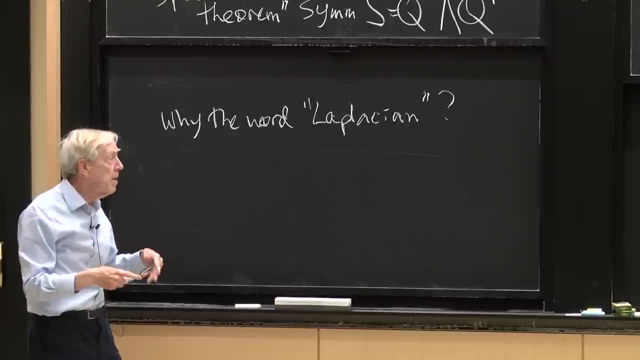 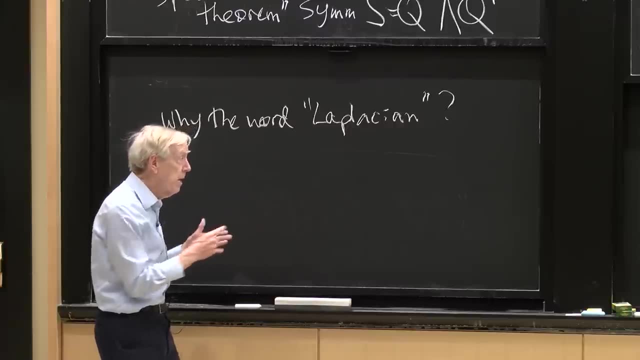 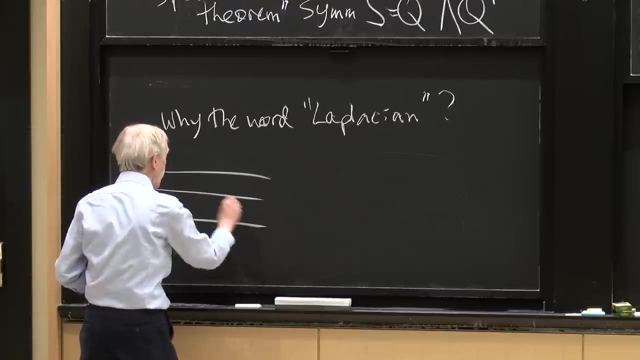 So the familiar thing. so it connects to Laplace's finite difference equation, because we're talking about matrices here and not derivatives, not functions, Yeah, So why the word Laplacian? Well, so if I have a regular, if my graph is composed of a, 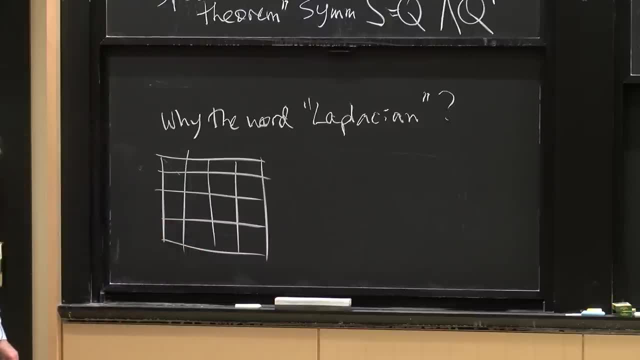 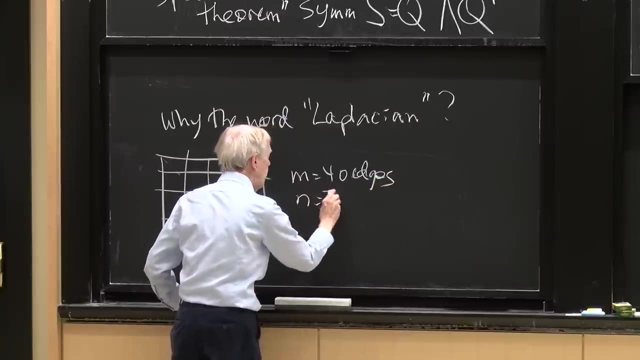 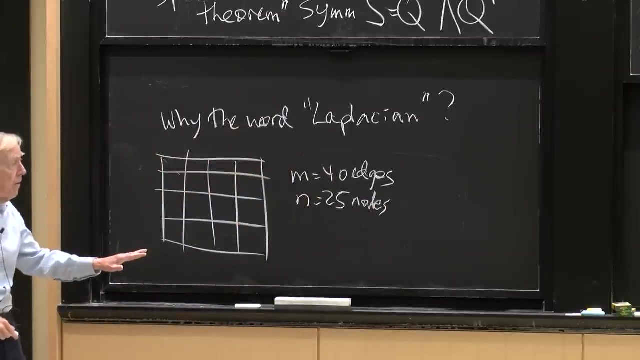 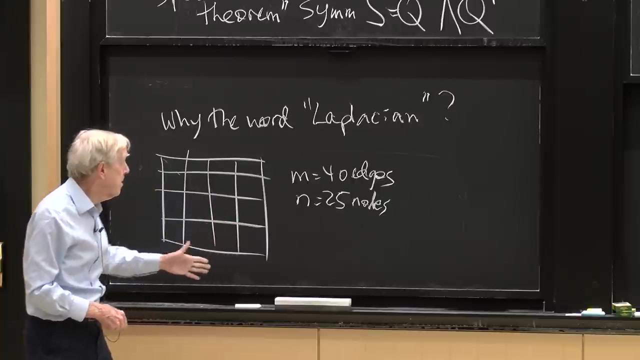 so there is a graph with 25 nodes and 4 times 5, 20, about 40.. This probably has about 40 edges and 25 nodes And of course I can construct its graph, all those four matrices for it: its incidence matrix, its degree matrix. 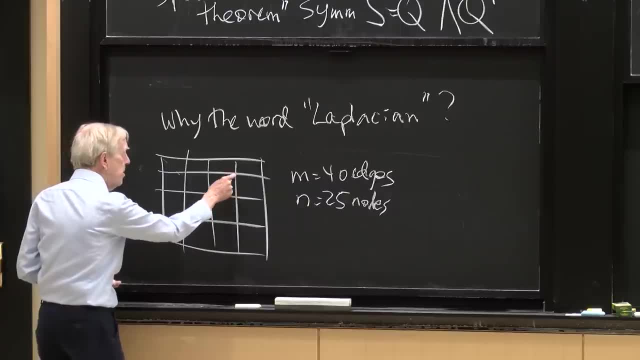 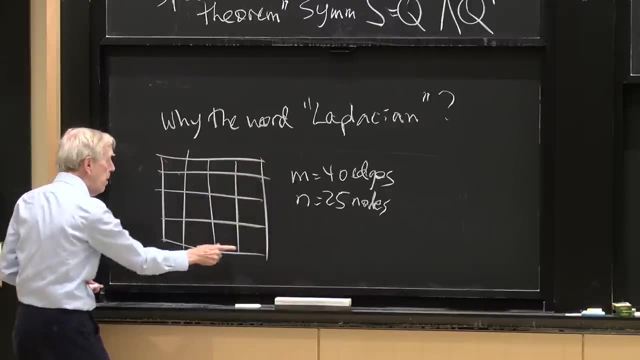 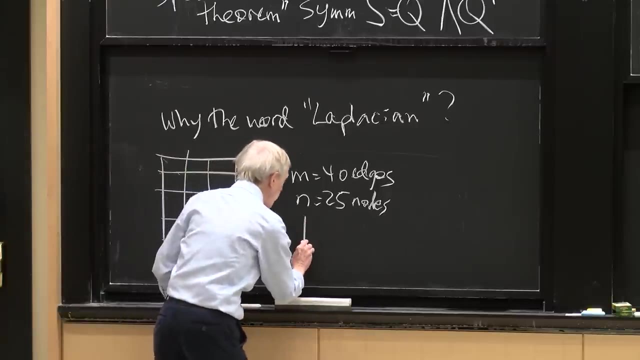 So the degree will be 4 at all these inside points. The degree will be 3 at these boundary points. The degree will be 2 at these corner points. But what will the matrix L look like? Yeah, So what is L? 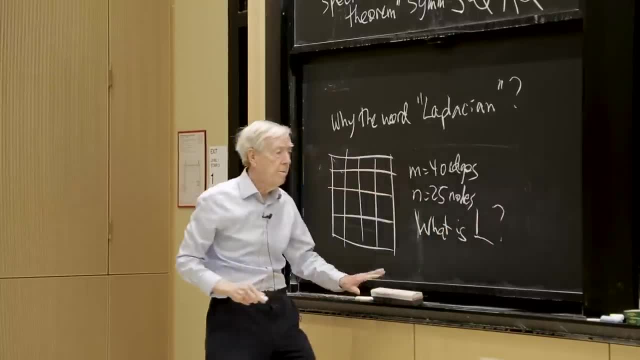 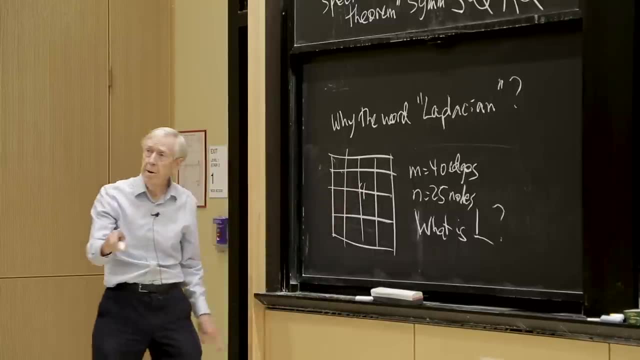 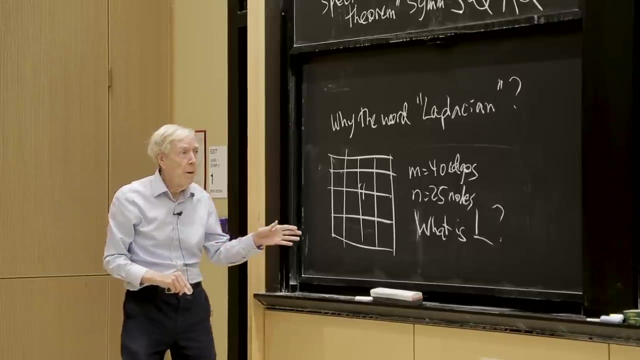 And that will tell you why it has this name: Laplacian. So the matrix L will have the degree 4, right will be on the diagonal, That's coming from D, The other, the minus 1's, that come from B. 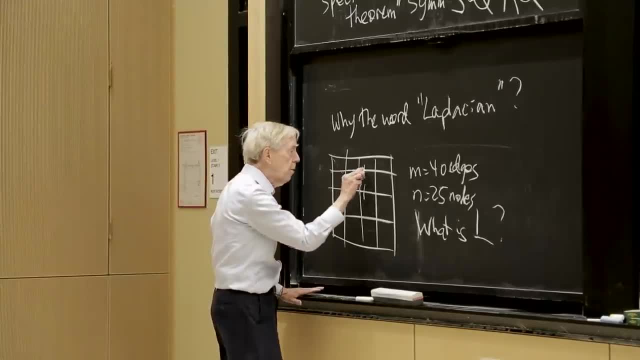 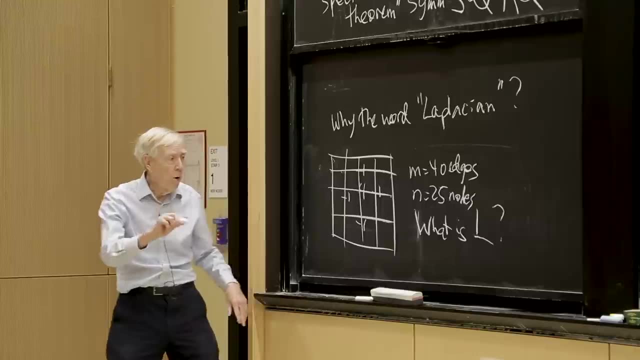 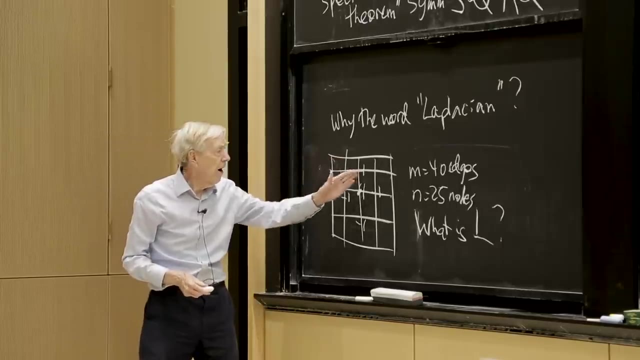 the adjacency matrix will be associated with those nodes And otherwise all 0's. So this is a typical row of L. This is a typical row of L centered at that node, So maybe that's node number 5, 10, 13.. 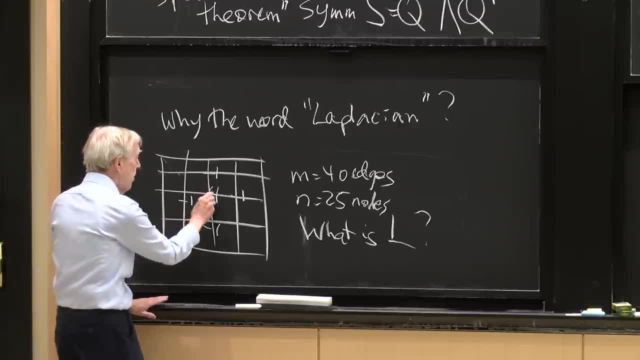 That's 13 out of 25 that would show you this And the sorry those are minus 1's, Minus 1's. So a 4 on the diagonal and 4 minus 1's. That's the. 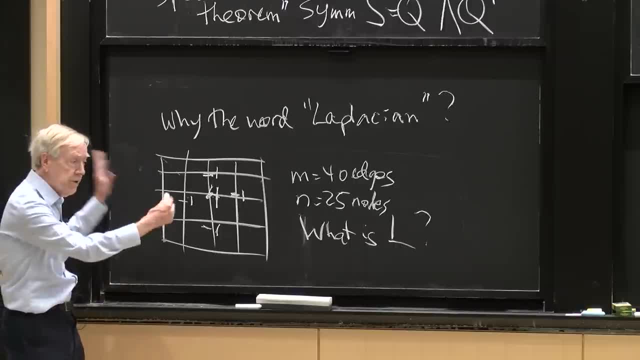 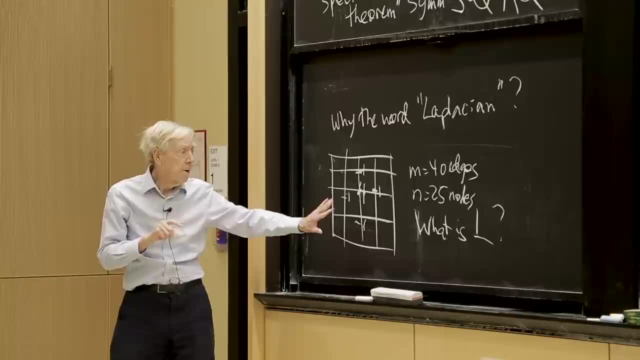 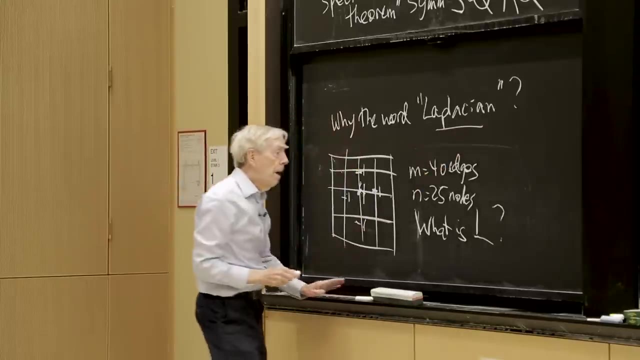 OK, That's the model problem, for when the graph is a grid, square, grid, And you associate that with Laplace's equation. So this is the reason that Laplace, why Laplace gets in it, Because Laplace's equation, the differential equation, 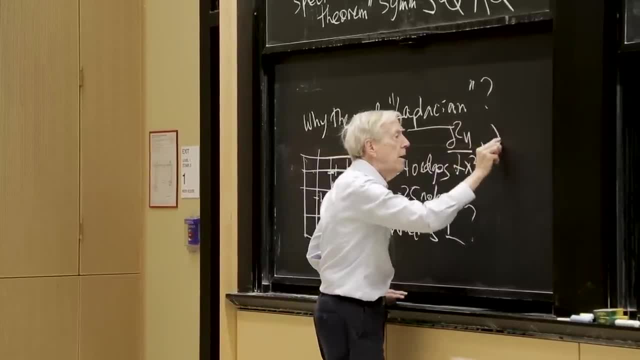 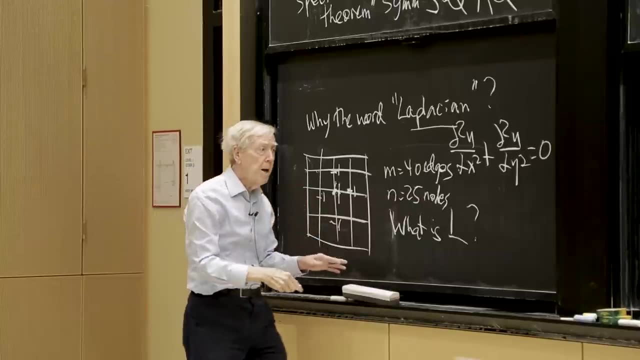 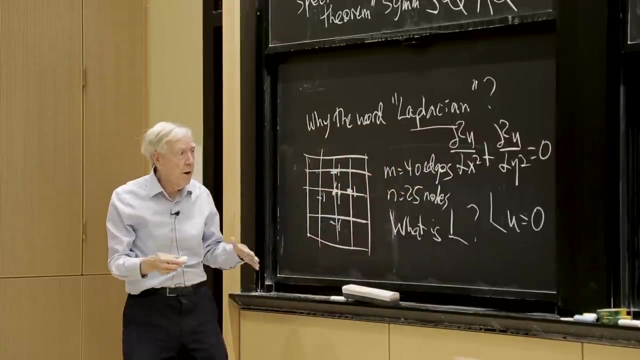 is second derivative with respect to x squared And the second derivative with respect to y squared is 0.. OK, And what we have here is L? u equals 0.. It's the discrete Laplacian, the vector Laplacian, the graph Laplacian, where the second x derivative is replaced. 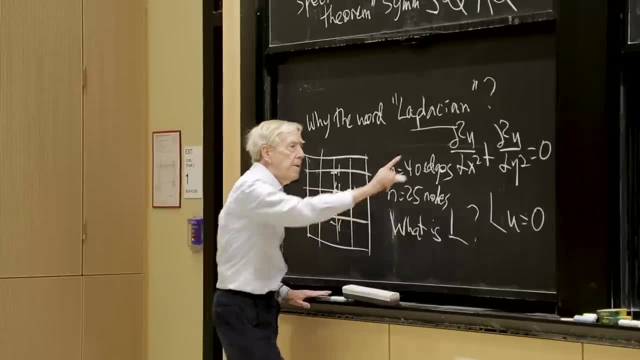 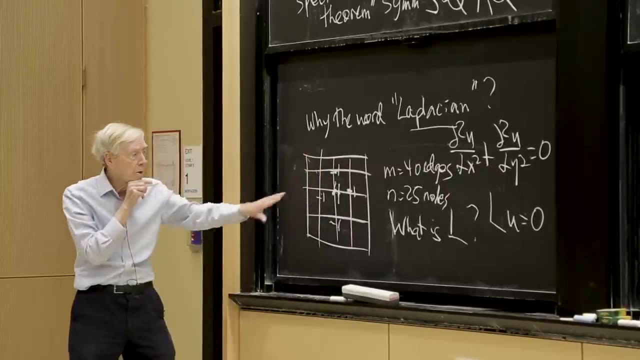 by minus 1,, 2, minus 1.. And the second y derivative is replaced by minus 1,, 2, minus 1.. Second: differences in the x and the y directions. So that's Yeah, Yeah, So. 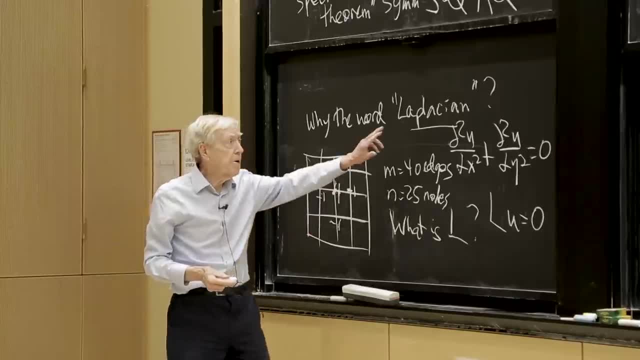 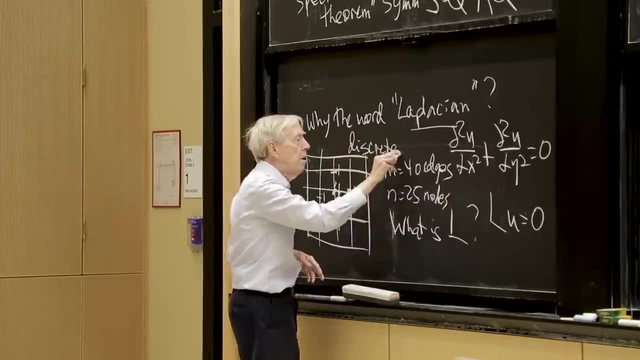 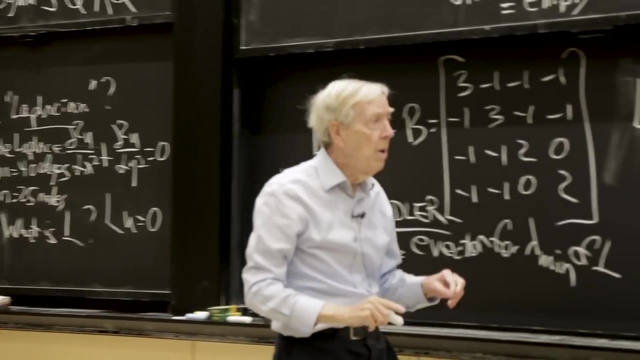 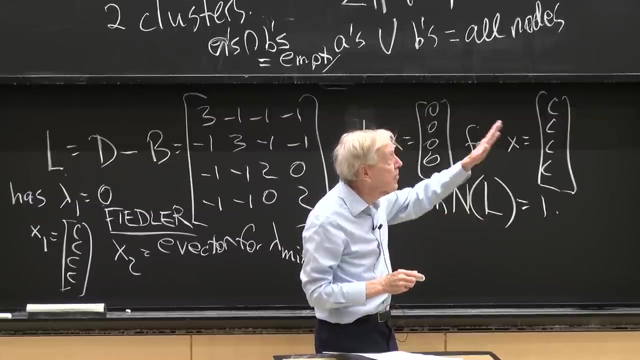 Yeah, Yeah, Yeah. So that's the explanation for Laplace. It's the discrete Laplace. Discrete or the finite difference Laplace. OK, Now to finish, I have to tell you what clusters. How do you decide the clusters from L? 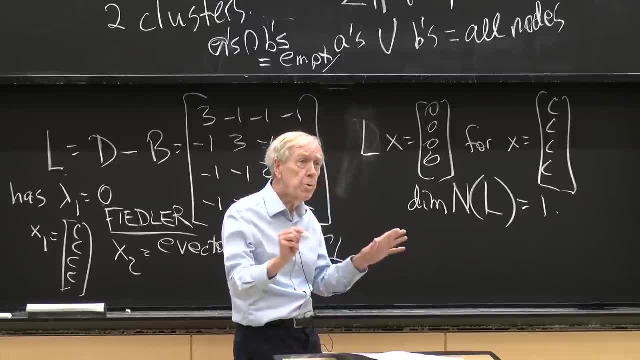 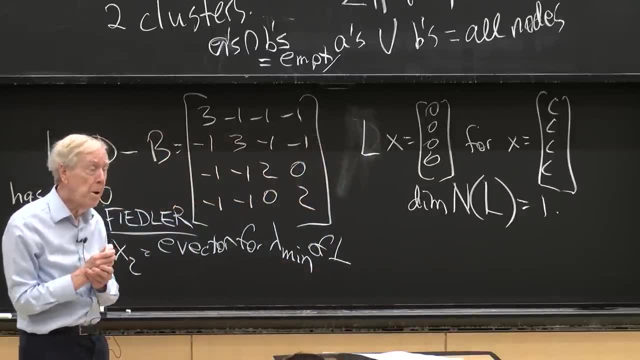 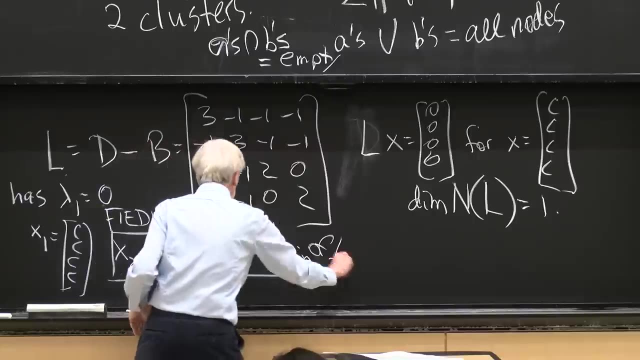 How does L propose two clusters, the a's and the b's? How does L propose two clusters, the a's and the b's? And here's the answer: They come from this eigenvector, the Fiedler eigenvector. 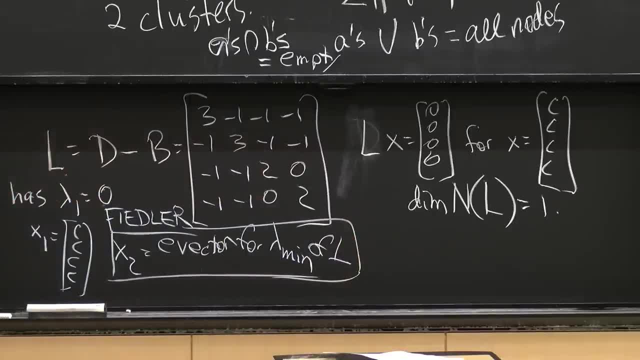 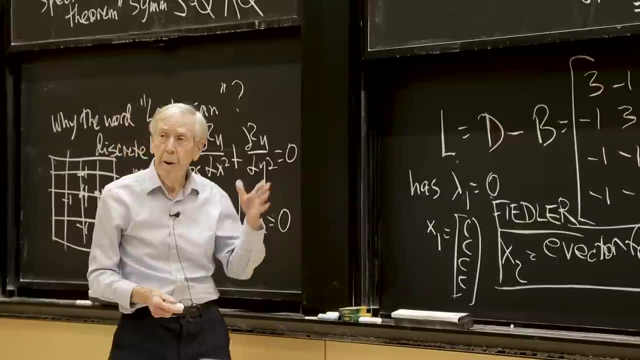 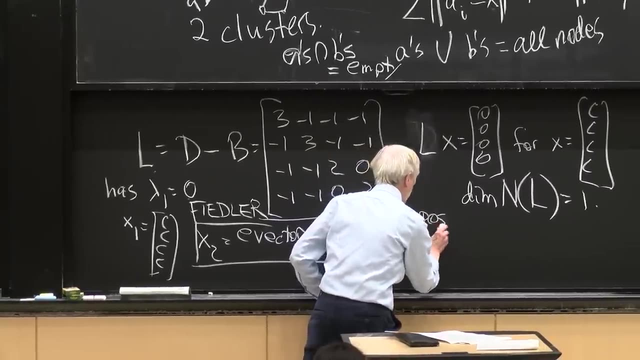 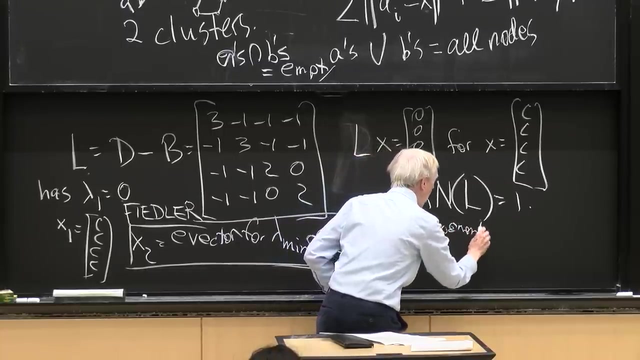 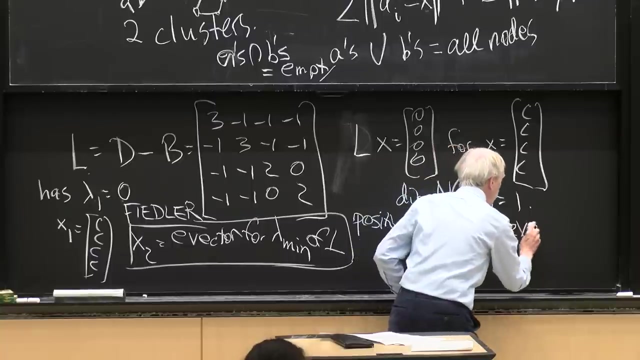 You look at that eigenvector, it's got some positive and some negative components, The components with positive numbers of this eigenvector. so the positive, The positive, The positive, The negative components of x of this eigenvector, and there are negative components. 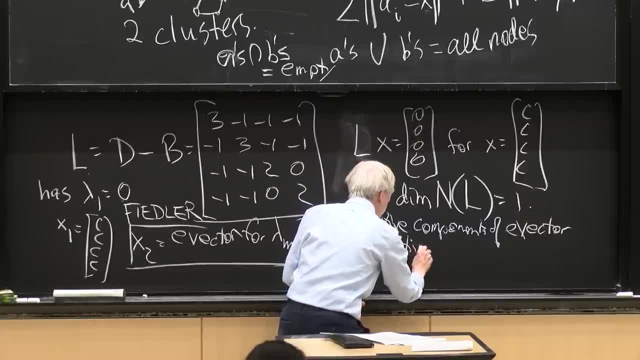 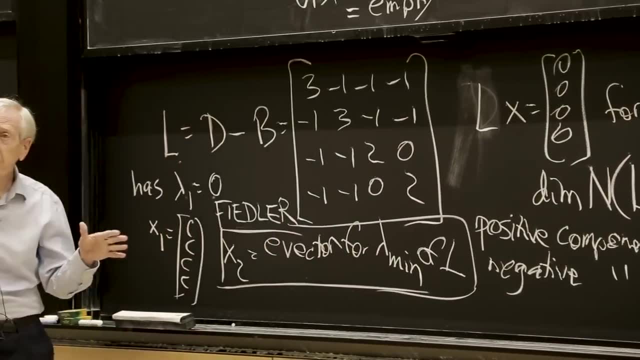 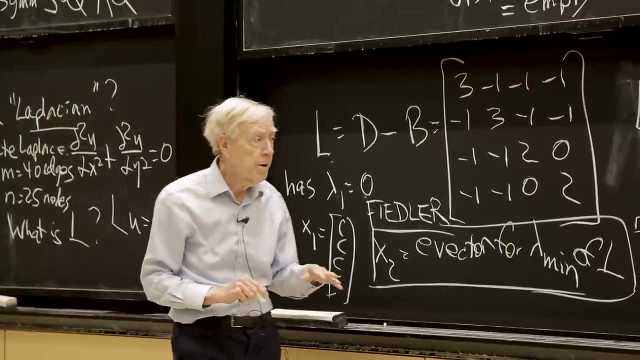 of this eigenvector And those are the two clusters. So the cluster is, the two clusters are decided by the eigenvector, by the signs- plus or minus signs- of the components. The plus signs go in one and the minus signs go in another. 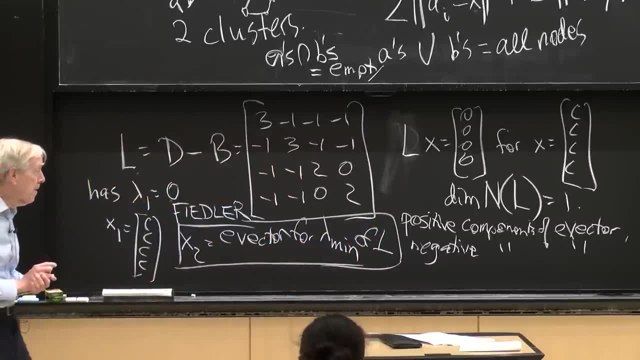 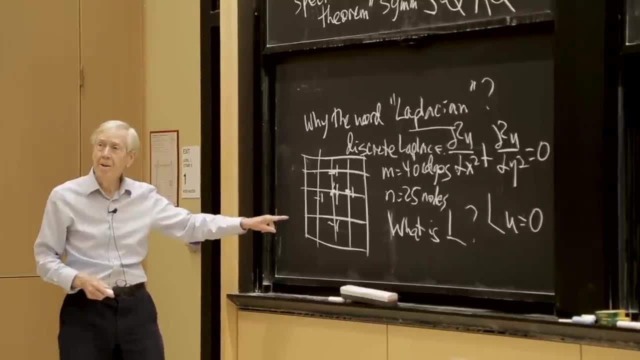 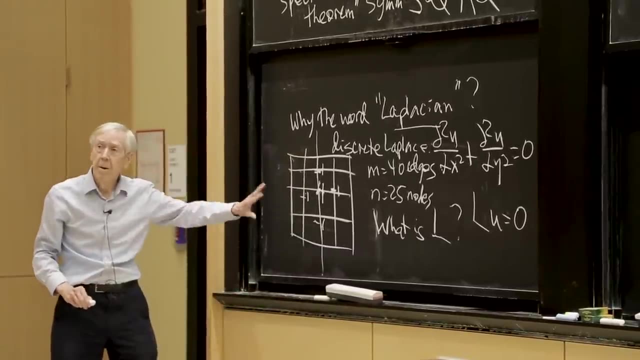 And you have to experiment to see that that would succeed. I don't know what it would do on this, actually, because that hardly splits up into two. I suppose maybe the split is along a line like that or something to get- I don't know what- clustering. 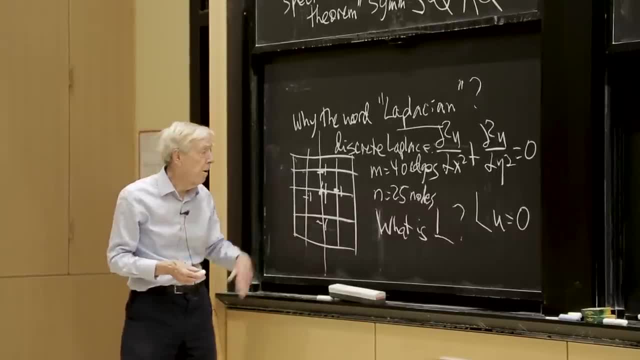 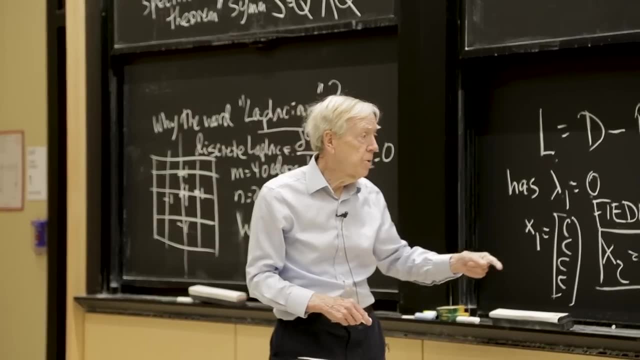 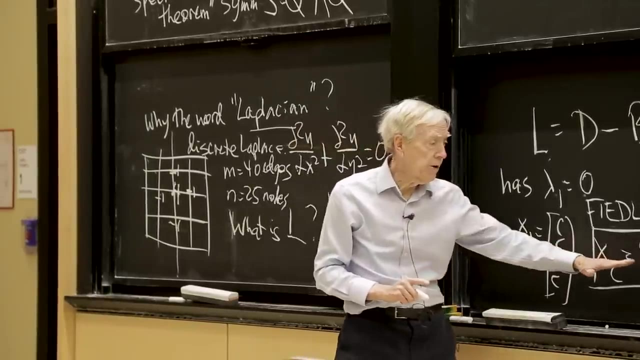 This is not a graph that is naturally clustered, But you could still do k-means on it, You could still do spectral clustering And you would find this eigenvector. Now, what's the point about this eigenvector? I'll finish in one moment. 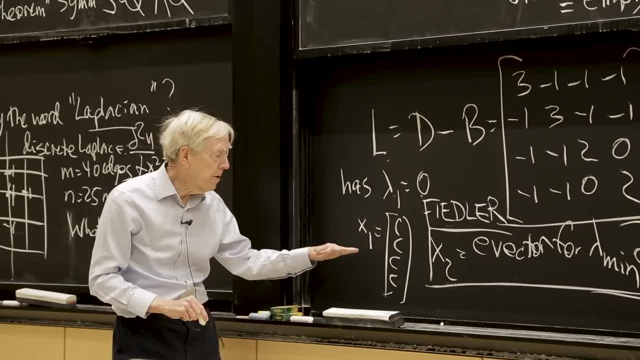 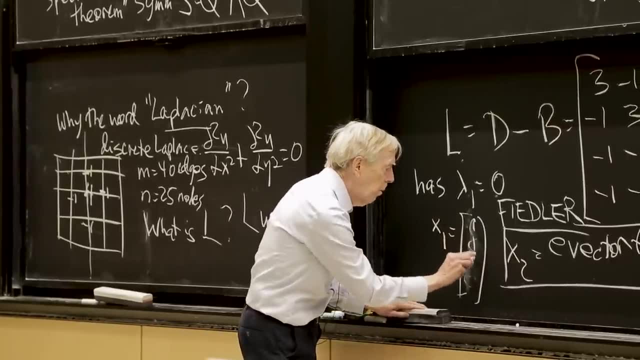 What do we know about that eigenvector as compared to that one? So here was an eigenvector, All 1's. Let me just make it all 1's, 1,, 1,, 1, 1.. In that picture it's 25 1's. 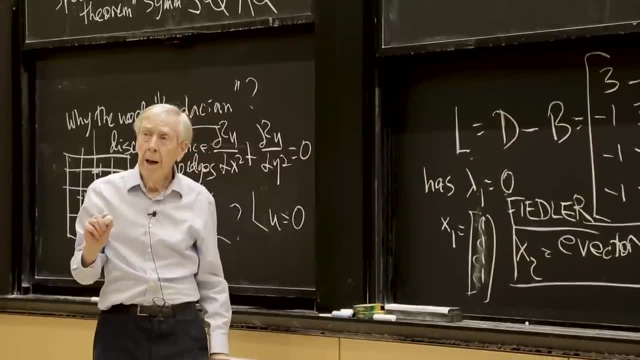 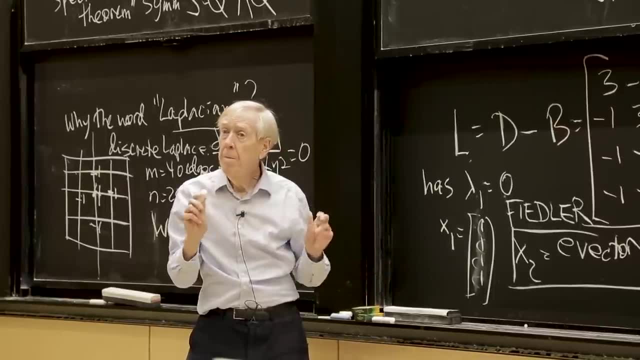 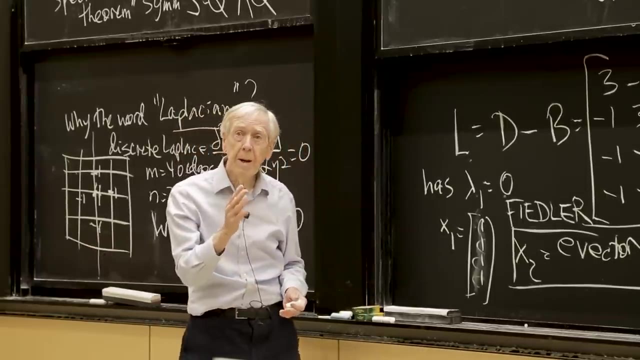 Here's the next eigenvector up. And what's the relation between those two eigenvectors of L? They are orthogonal. These are eigenvectors of a symmetric matrix, So they're orthogonal. So that means to be orthogonal to this guy. 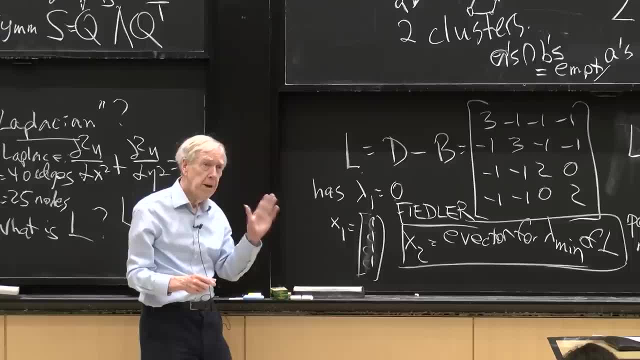 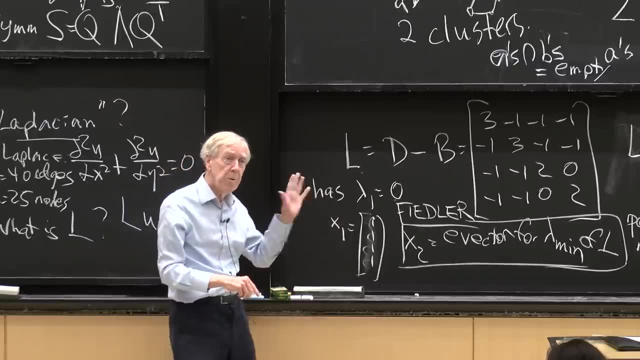 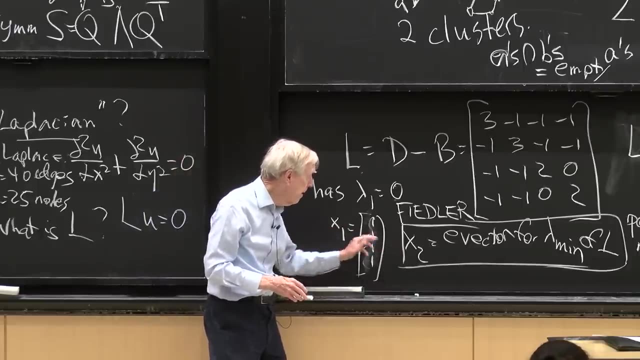 means that your components add to 0,. right A vector is orthogonal to all 1's. That dot product is just add up the components. So we have a bunch of positive components and a bunch of negative components. They have the same sum because the dot product with that. 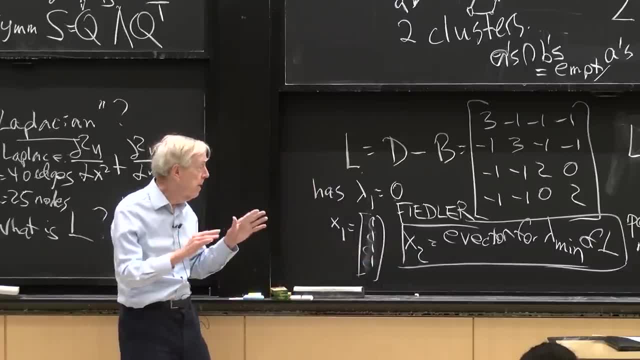 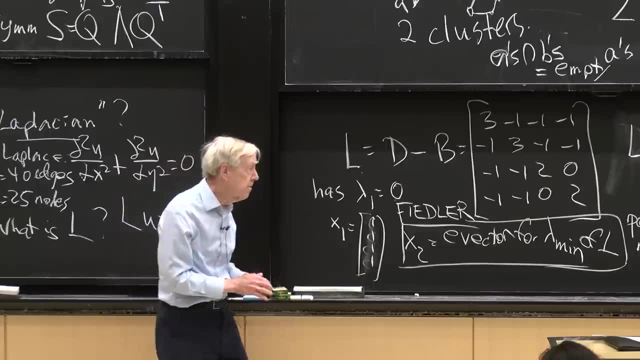 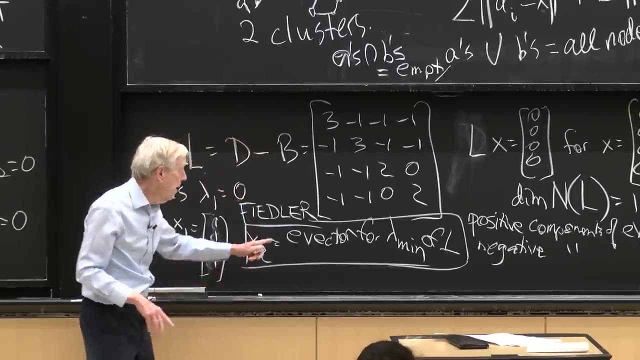 is 0. And those two components, those two sets of components, are to tell you the two clusters in spectral clustering. So it's a pretty nifty algorithm. It does ask you to compute an eigenvector And that, of course, takes time. 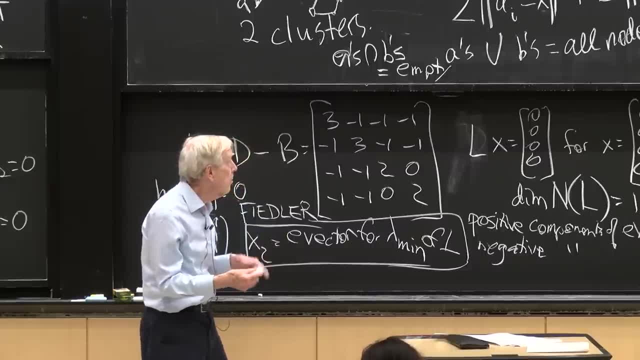 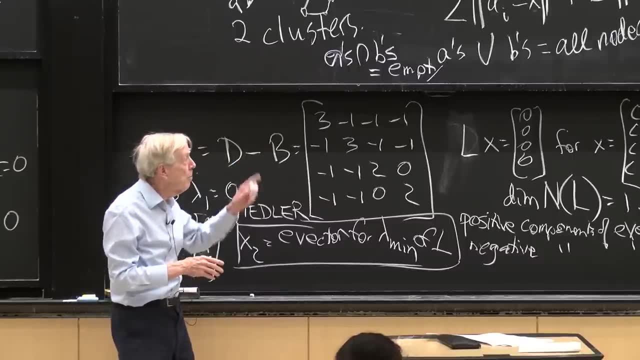 And then there's a third, more direct algorithm to do this optimization problem. Well, actually there are many. This is an important problem. So there are many proposed algorithms. Good, OK, I'm closing up. Final question: Yeah, 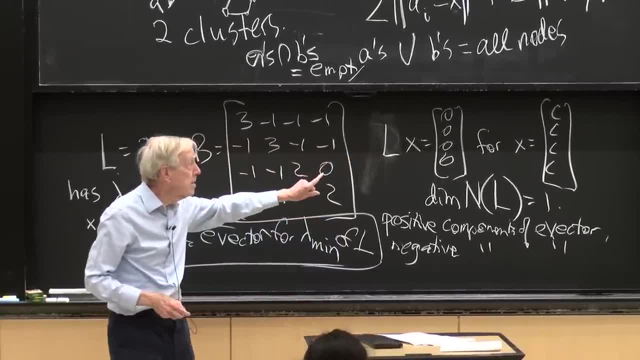 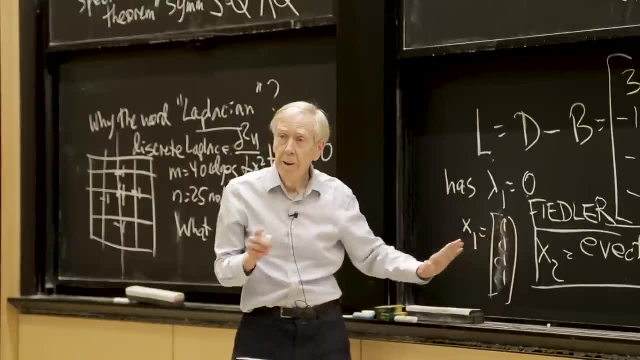 Could it be more than one eigenvector? GILBERT STRANG- Well, certainly for k-means. Now, if I had to do three clusters with Fiedler, I would look at the first three eigenvectors. Well, the first one would be nothing. 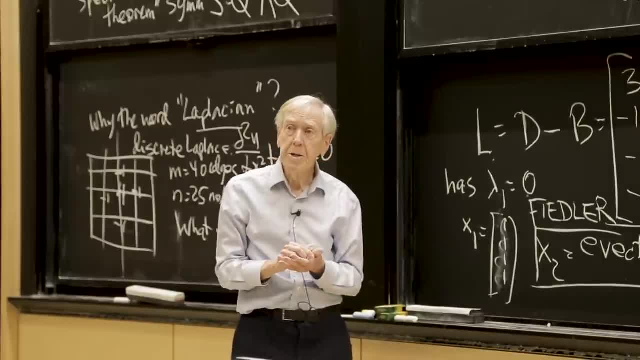 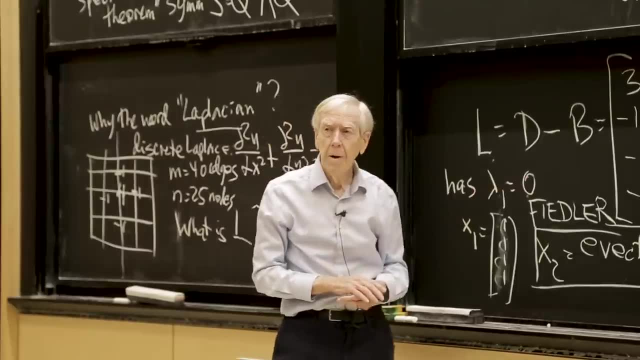 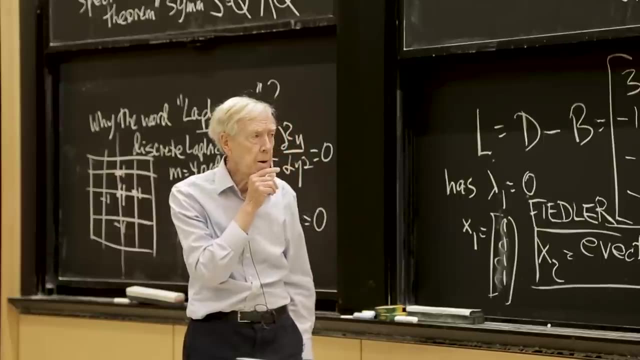 And I would look at the next two And that would be pretty successful. If I wanted six clusters it probably would fall off in the quality of the clustering. Yeah, but certainly I would look at the lowest six eigenvectors And get somewhere. 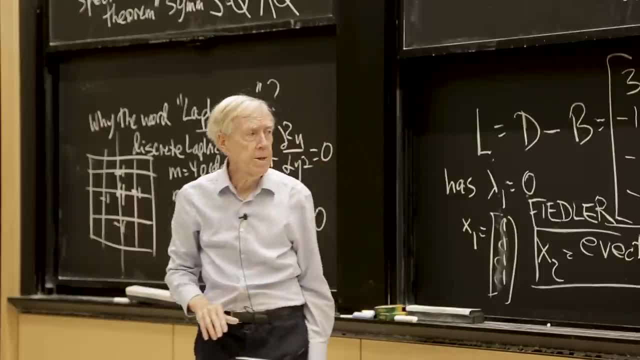 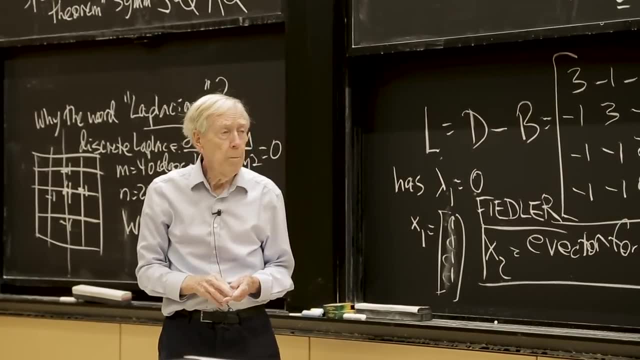 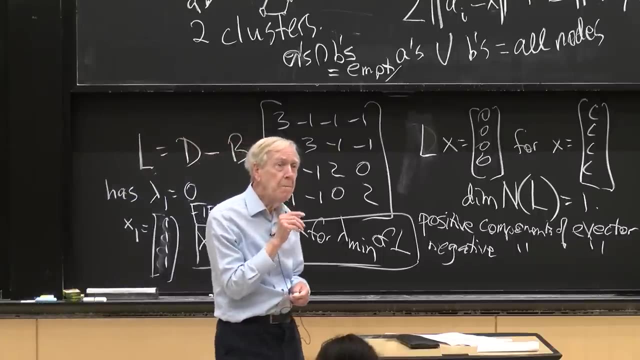 Yeah, right, So OK. so that's a topic, an important topic, a sort of standard topic in applied graph theory. OK, so say you're Wednesday, I'm hoping, I'm hoping on Wednesday. so Professor Edelman has told me a new and optimal way. 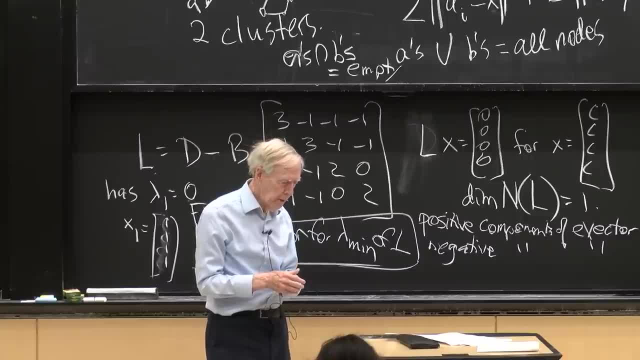 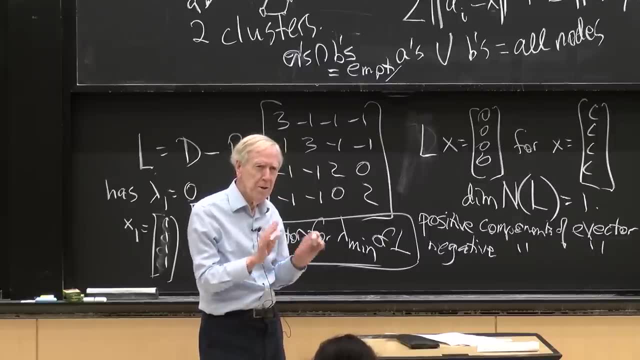 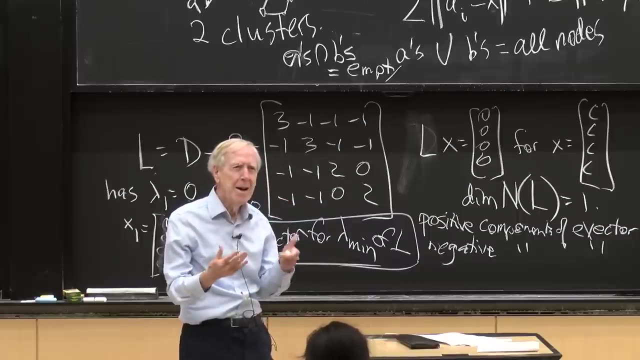 to look at the problem of back propagation. You remember back propagation. If you remember the lecture on it, you don't want to remember the lecture on it. It's a tricky messy thing to explain. But he says: if I explain it using Julia in linear algebra: